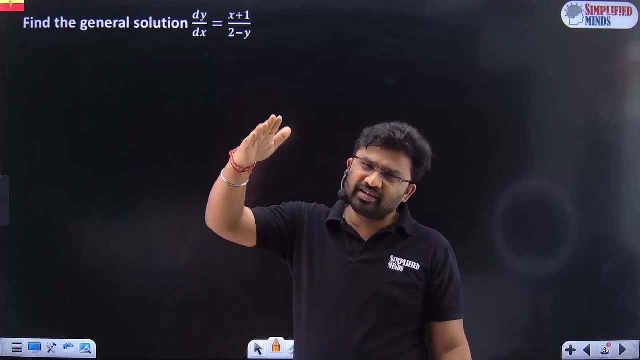 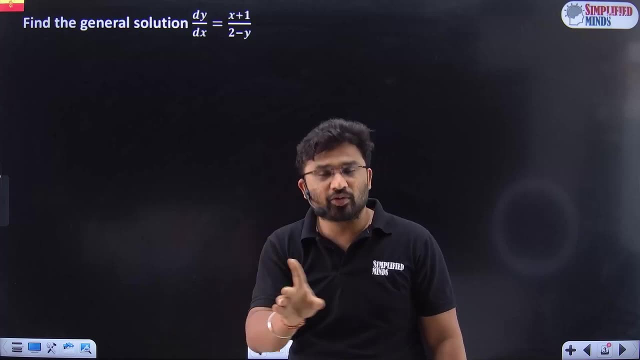 Because methods of solving is just an addition And anyway, almost 90% integration is there. Only the starting 2-3 steps are different. You should know the entire integration chapter. You should know all the methods. This is very, very important. 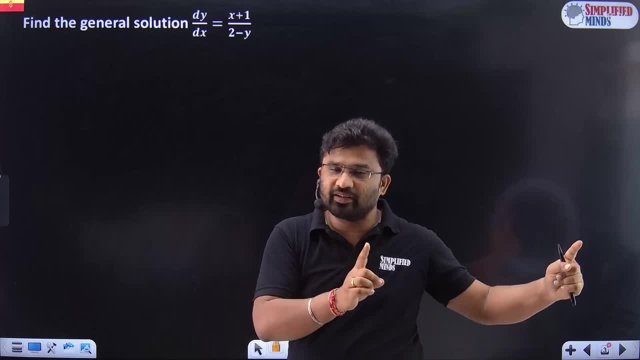 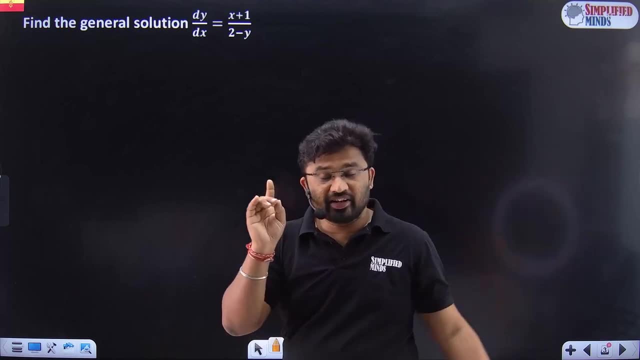 I have already completed it. What is the beginning? I think only 8 hours is there mostly. I think only 8 hours is there mostly. I have completed the entire integration Only. if you know the integration well, you should watch the differential equation lectures. 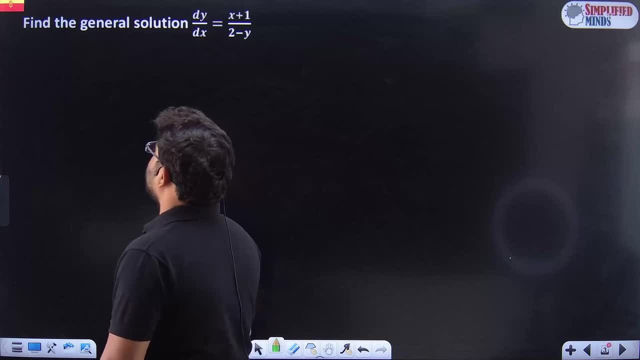 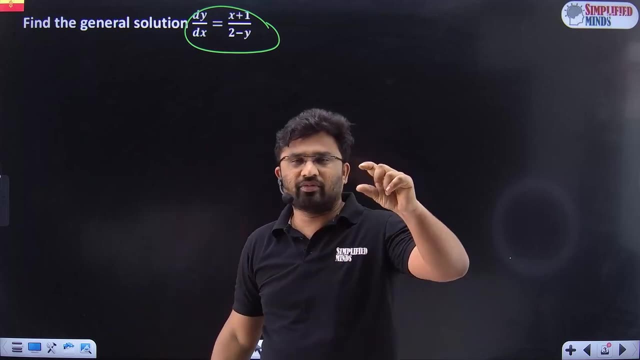 Because it will be very easy for you. It will be very easy for you. The first method, as the word says: Variable, Separable. What we have to do is: y is equal to f of x. I have already told you in the previous lecture. 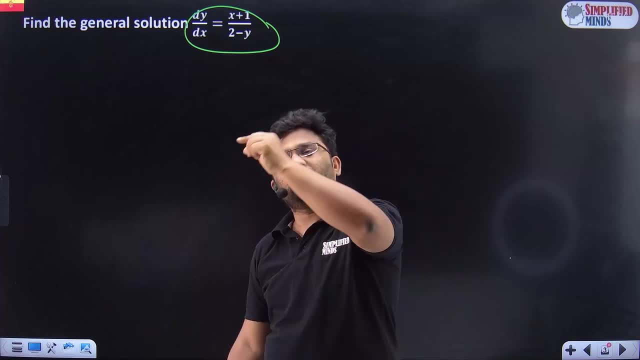 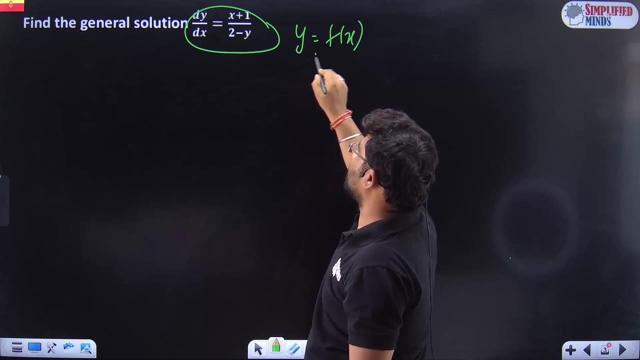 y is equal to f of x. After differentiating it, we will get the differential equation. After integrating it, we will get the solution. The solution of the differential equation is: y is a function of x. I have explained everything in the previous lecture. 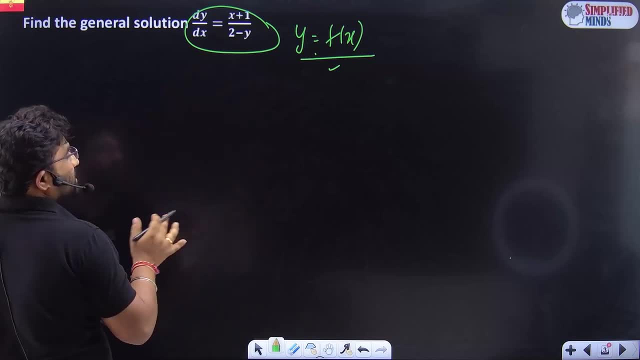 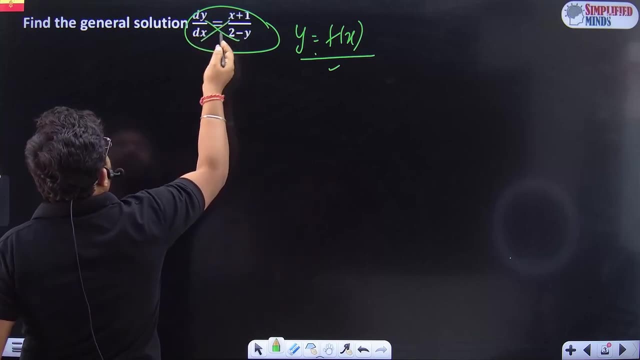 I have explained everything in the previous lecture. First, what we have to do is Variable Separable, Separate the variables All x is one side and y is one side. We will do cross multiplication dy into 2 minus y, dy into 2 minus y. 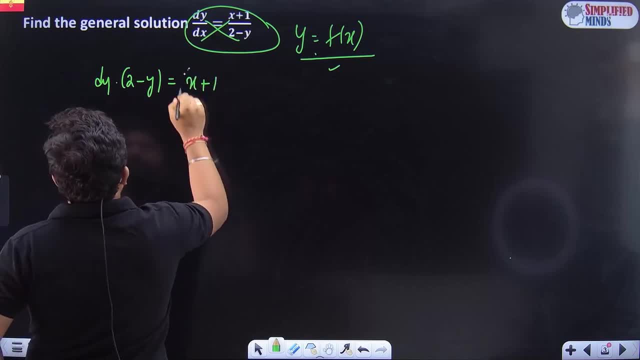 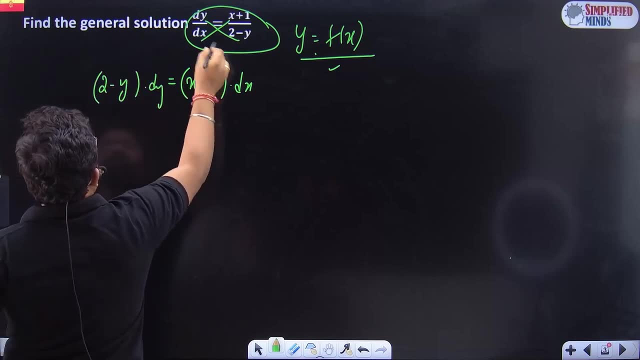 should be equal to x plus 1 into dx. x plus 1 into dx- It is difficult to shift like this. Very simple 2y into dy is equal to x plus 1 into dx. That is why we have to integrate. 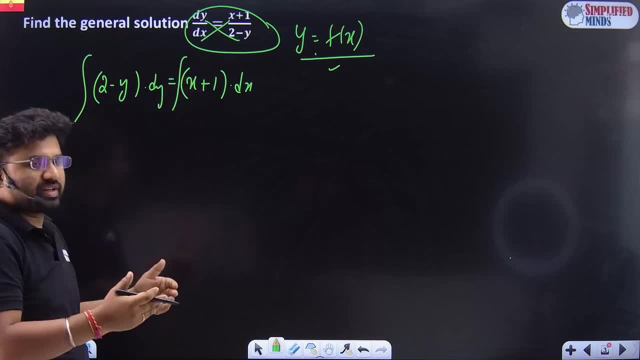 It is simple: Every method, whether it is linear or homogeneous, whatever method you learn in the future, there will be a difference of two steps. Everything is integration. That is why we have to be an integration expert. We have to know all the methods of integration. 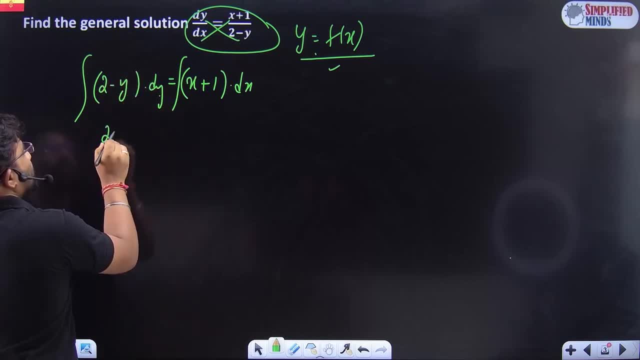 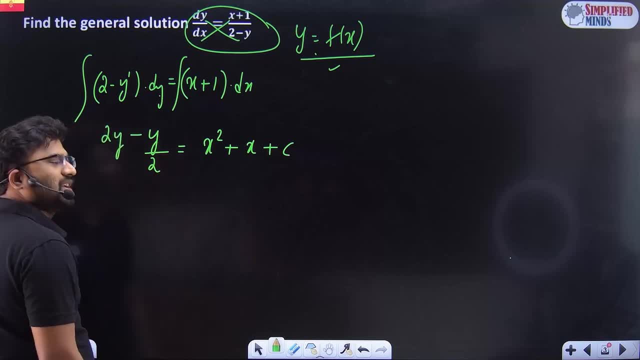 dy into dy is: dy is: dy is 1 plus 1 divided by dy into dy is 1 plus 1 divided by 1 plus 1. that is y square. That must be equal to integration of x square where 1 for 1 is 1x. 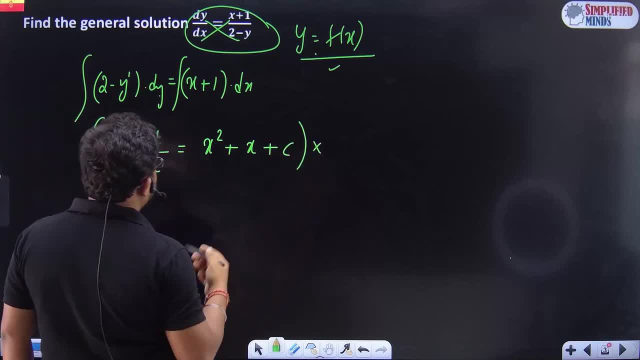 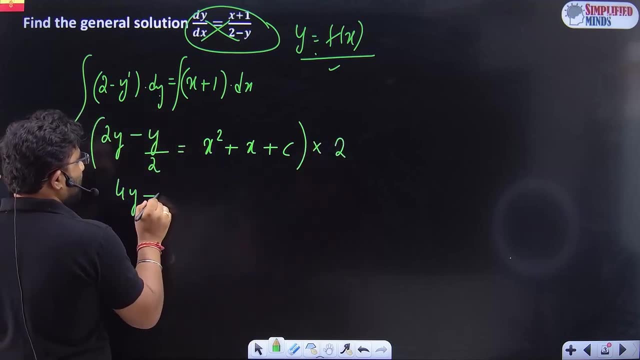 so it is basically x plus c. Do we have to have C on 2 sides? It is not required, but it israconstant answer we will get. the answer is four y minus y, two x square plus two, x, three plus two c entire. 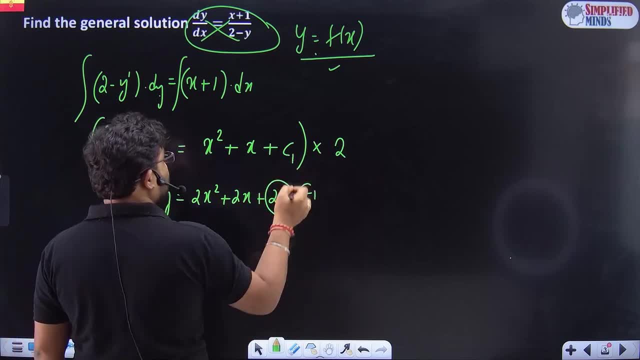 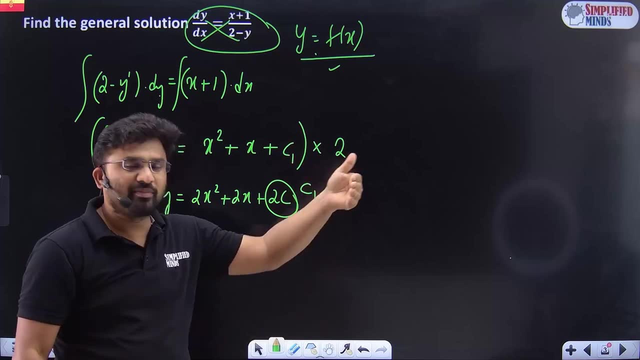 if you want, you can again make it as something like c1 or it didn't see one, though we didn't see him, so don't worry about especially integration constants. now, if you are the baker tommorow then you can. examples: only: integration constant. log c to home tv. 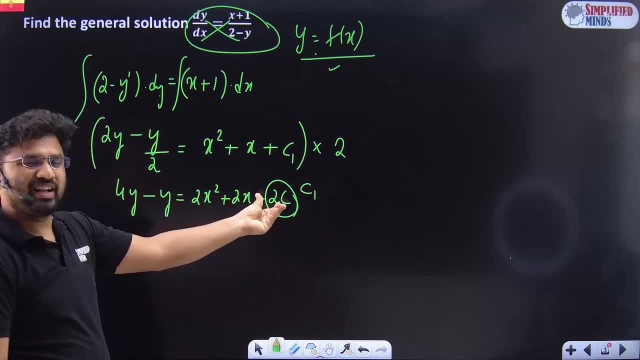 elements are: e power, c to home tv. so, depending on the question, we can take whatever we want: integration constant, i'll try it up. so you got four y sorry, uh. four y minus y. yeah, oh, why it became sorry y square, y square. and four y minus three y. out there one on your time. 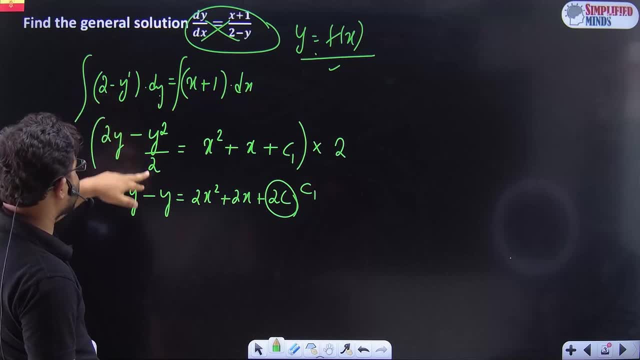 so two into y and y, l will breathe. okay, y square divided by two and a lot to multiply model: get the four: y minus y. y square minus y square is equal to x plus 2c plus c is the answer, r plus c1 is the answer. so variable, separable. 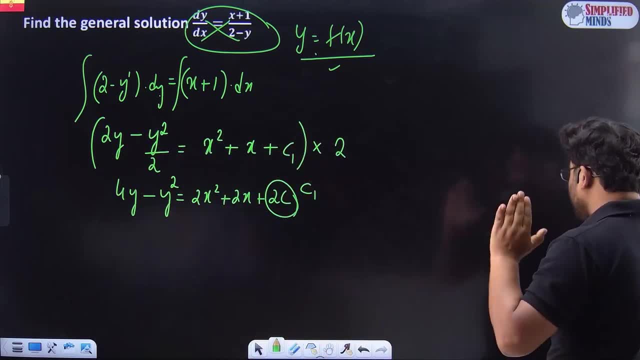 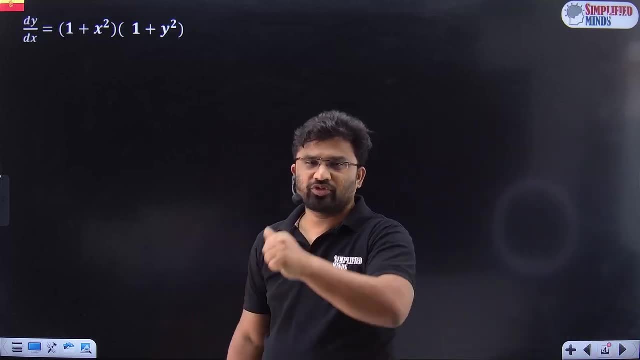 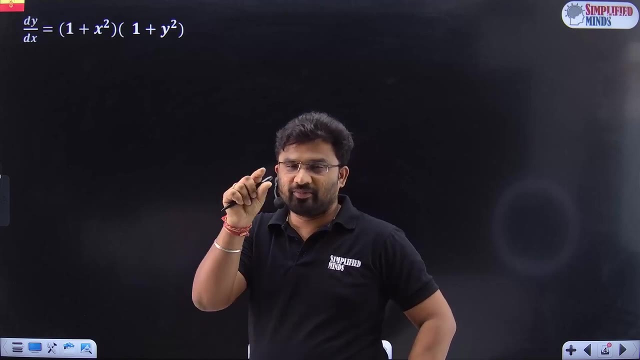 now variables are separate. mark onto integrate model could know by easy. it's very, very easy, not not only board examily, they can ask a simple question, so most of the time question the linear material character, five markers together so it really could have three marker question character clinic drillins, the word question, keita, word problem, other than the learning and 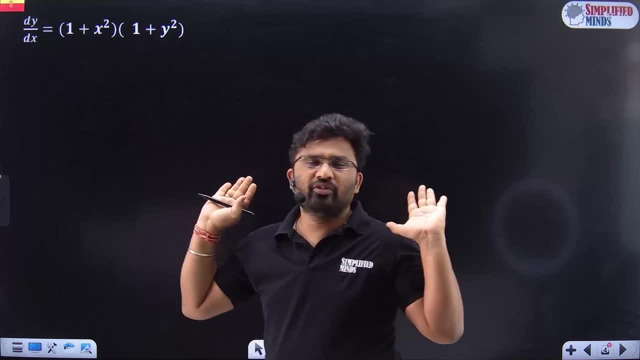 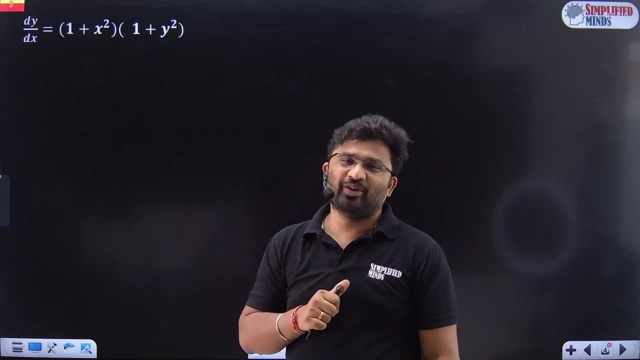 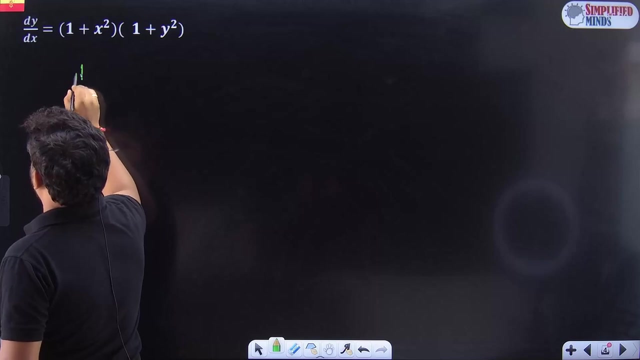 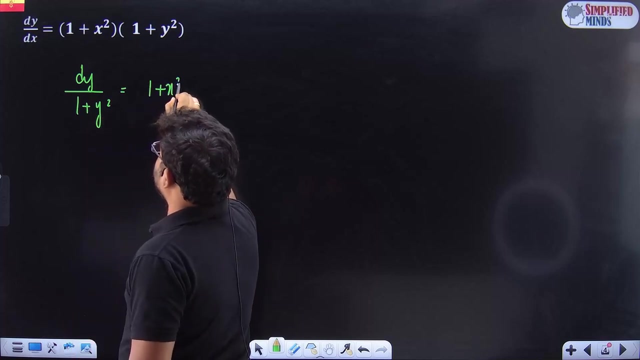 teacher. that also okay, it's very simple. next video again monitor video. pause modico integration. go to the hills could all all the lectures in order to re video. now pause money. you will solve. So d y divided by 1 plus y square must be equal to 1 plus x. square into d x. 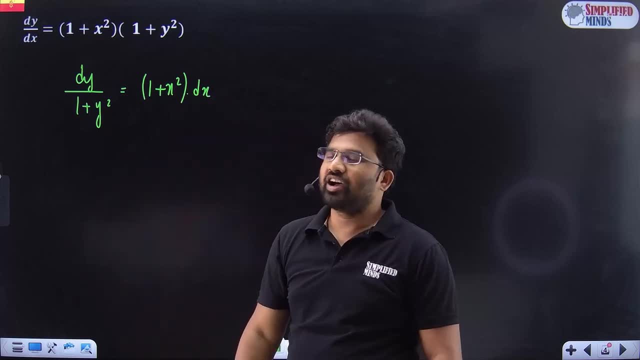 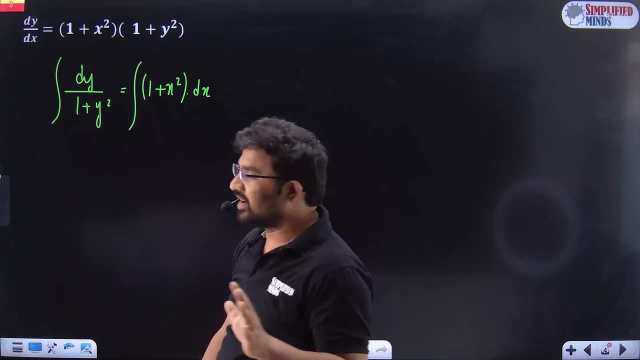 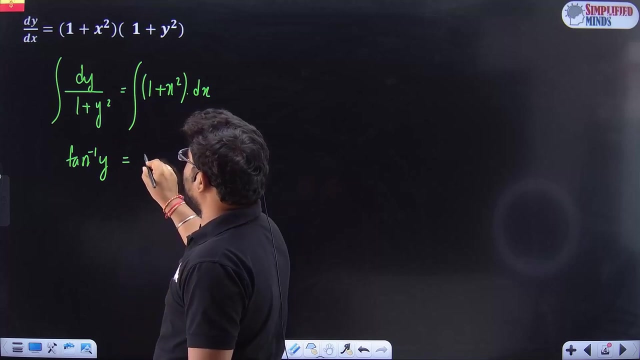 1 plus x square into d x, Integrate it. Integration of 1 divided by 1 plus y square is very famous. Tan inverse of y, Tan inverse of y. Integration of 1 divided by x. Integration of x divided by x. cube divided by 3 plus c. 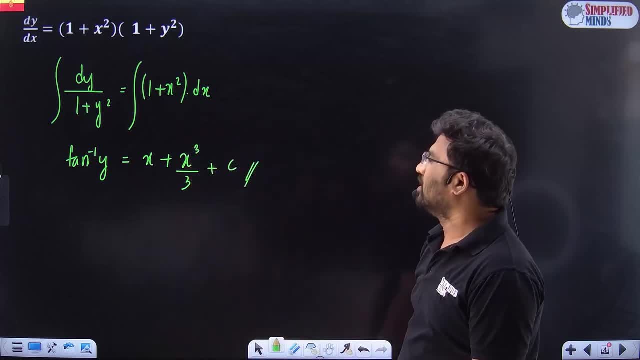 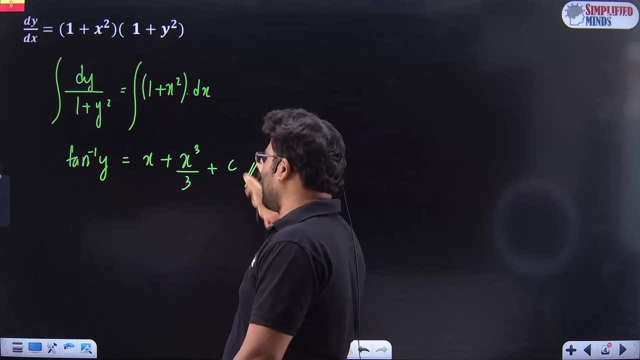 That's the answer, Easy, isn't it? Tan inverse of y is equal to x cube plus x plus x cube divided by 3 plus y. If you want to get y, bring tan this side: Tan of x plus x cube plus 3 plus y. 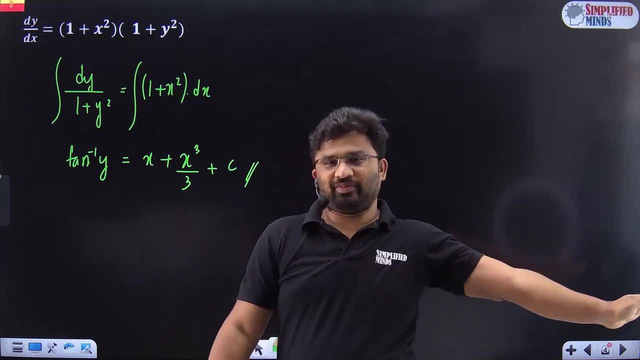 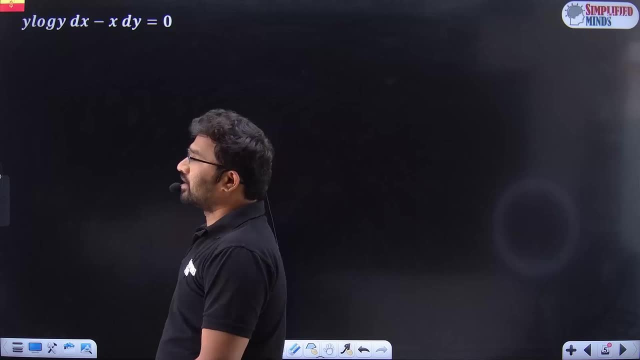 Simple, Variable. separable is the easiest method. All methods are variable. separable is the easiest method. If you have any more questions, you can ask them in the comment section, So every time you don't have to ask a direct question. 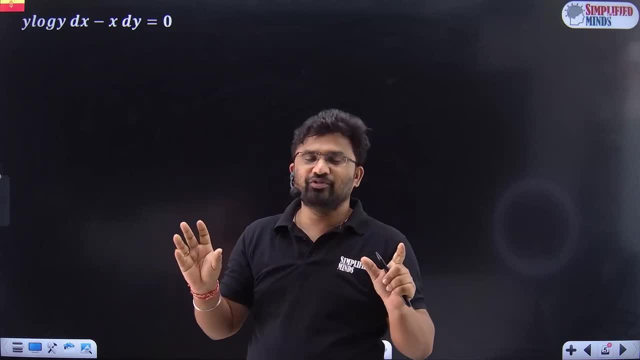 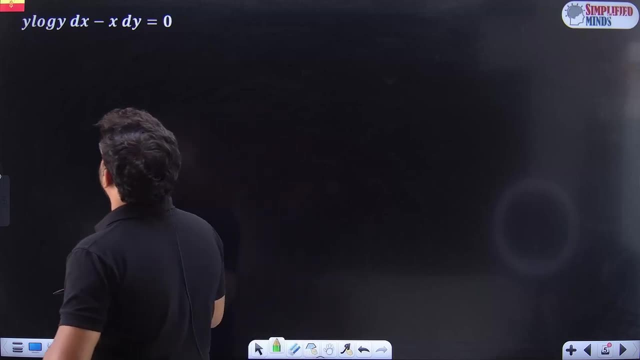 As you can see, it's not easy to get a variable separable, So you have to think: So first y into log y, d x is there, Minus x into d, y is there. So let's try to. 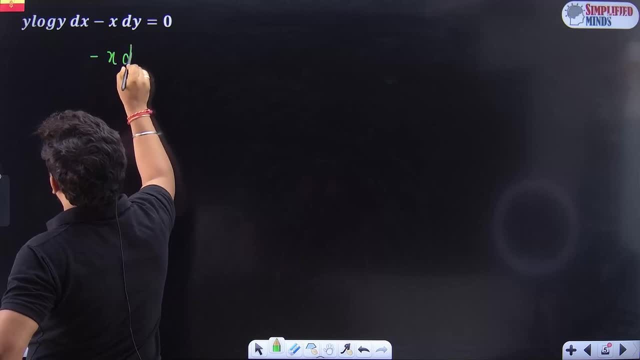 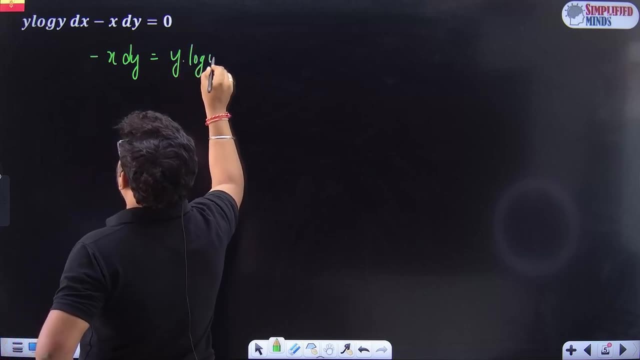 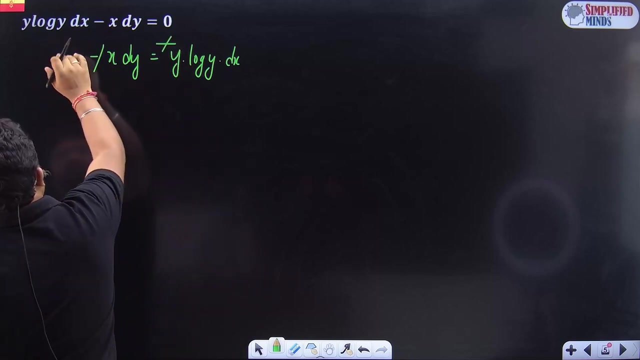 put d y here. If you put minus x d y here, I'll put y log y there, y log y, y log y into d x. So this is minus. So both minus and minus cancel. No, This goes here and this goes here. 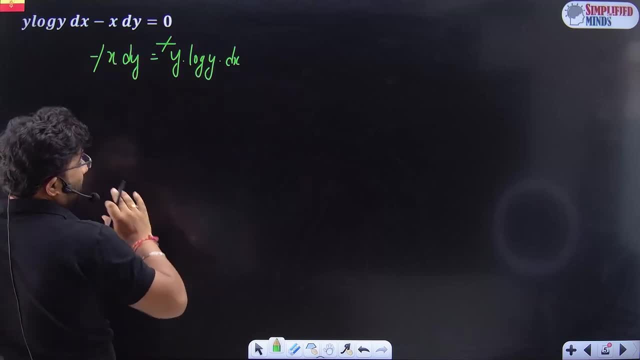 I just kept it like this because I wanted y to be equal to something. Do it both ways and you'll get the same answer. So what's next? Basically, we have to shift all the y's one term. We have to bring all y's to one side and all x's to one side. 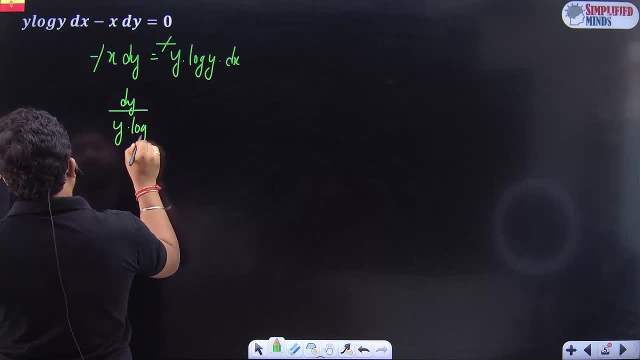 So d y is there? d y divided by y log y? What's here? d x divided by x? We have to integrate this. To integrate this, y log y is equal to 1 by x into d x. So how to integrate this. 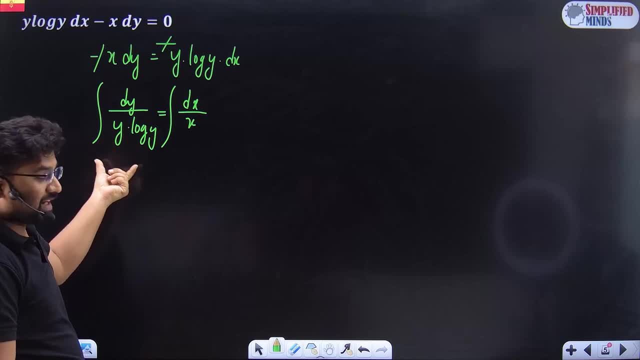 You need to know this. If you're not able to guess this, that means you haven't read the integration properly, The integration. So we can easily guess this: How to integrate y log y. What do we learn from integration? The first method is the substitution method. 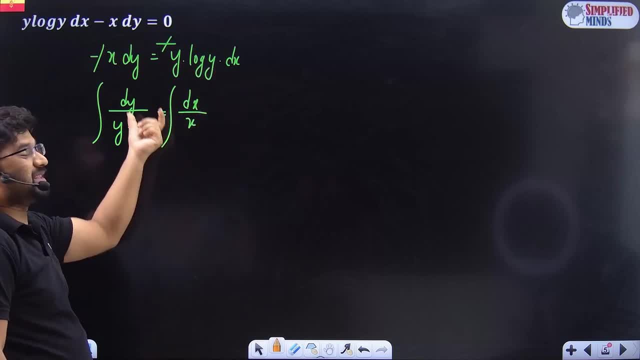 I asked so many questions in the substitution method, So you have to take something. We don't learn. integration of 1 by log y- much right Usually. So integration of 1 by y is log y, So log y is creating a problem. 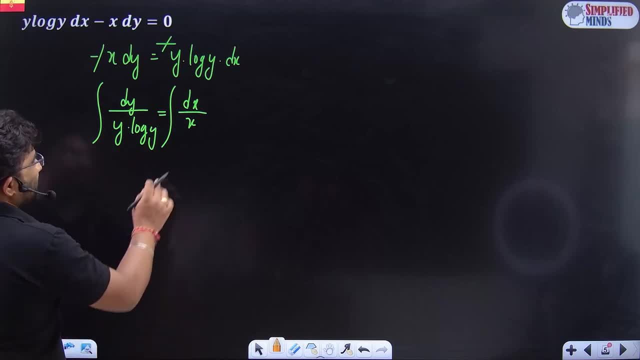 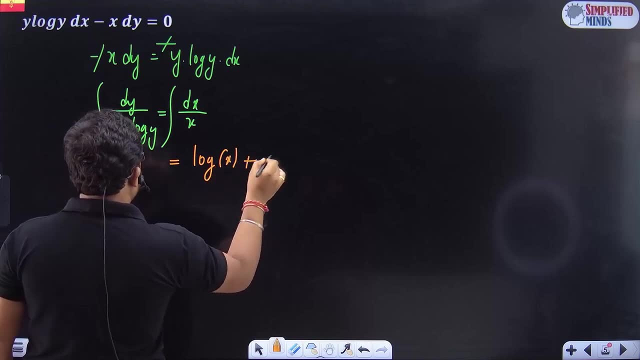 When a problem is created, it becomes t. See, this is the integration. When integration happens here, this becomes very simple. It becomes log x. I will write integration as plus c. When integration happens here, we have to integrate this. 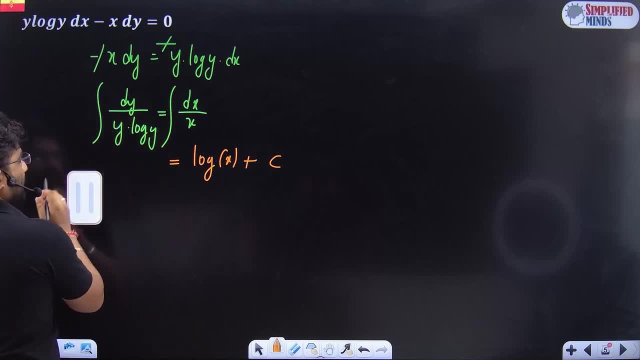 What I will do is to integrate this. let us take log y as t. I will take log y as t. What is the log y differentiation? 1 by y, 1 by y dy, That is dt, So dy by y. 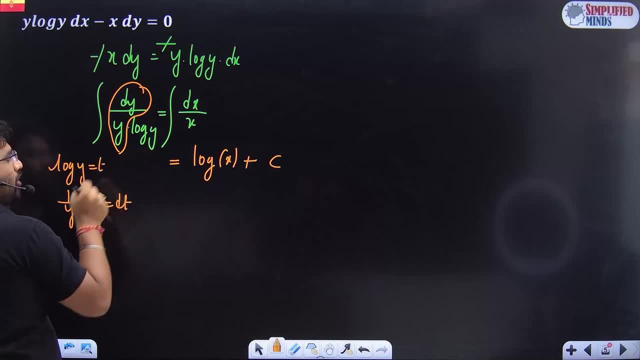 That becomes dy, by y becomes dt, Log y becomes t. What is log y? Basically, what is log y? It becomes t. So what is integration? Integration of 1 by t, dt is equal to okay, anyway. 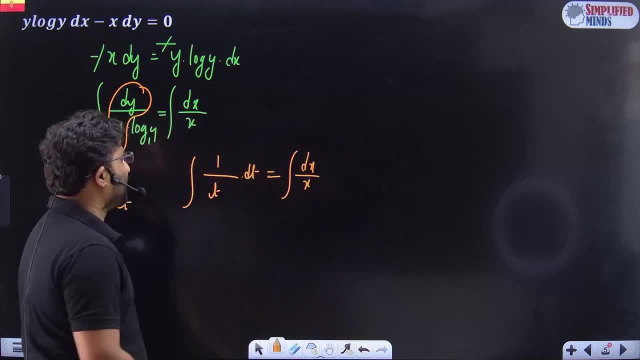 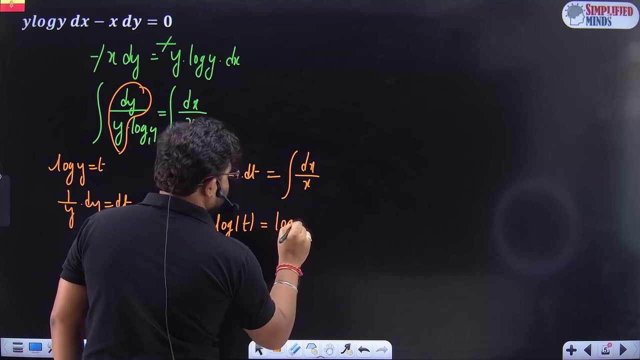 this is not simple: dx by x, Is that clear? So this is the method of substitution Integration. Integration is very important. What is integration of 1 by t? log t is equal to log x plus. So what to take? 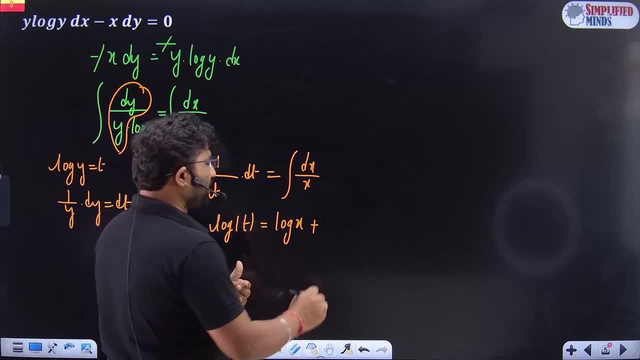 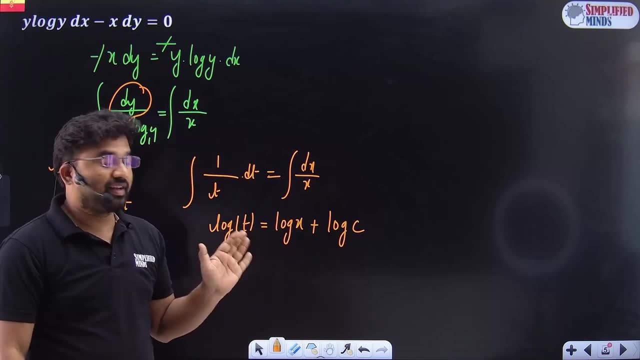 See, here all are logs. So to maintain uniformity, we can take log c. So what happens when we take c? No problem at all, No issue at all, Because this will give more simplified answer. What do you know? 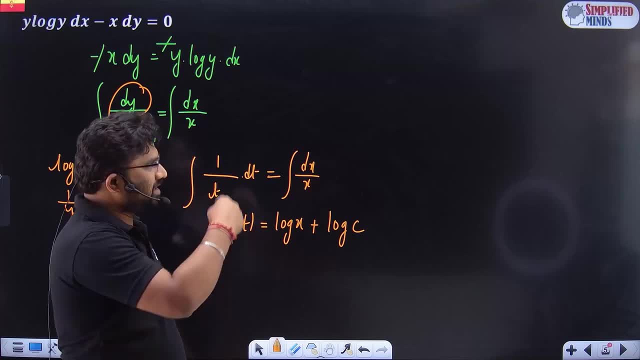 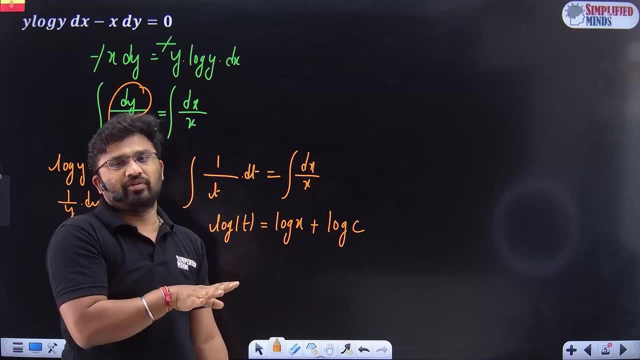 Actually, if you ask any question you will get the answer, Because I think some question is: x is equal to 1, y is equal to 1.. You have to calculate c. In actual, real problems. you have to calculate c. 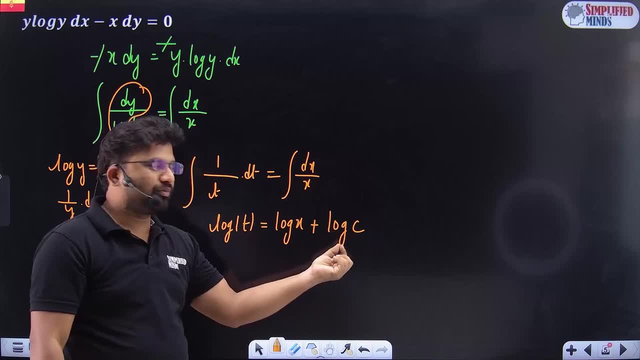 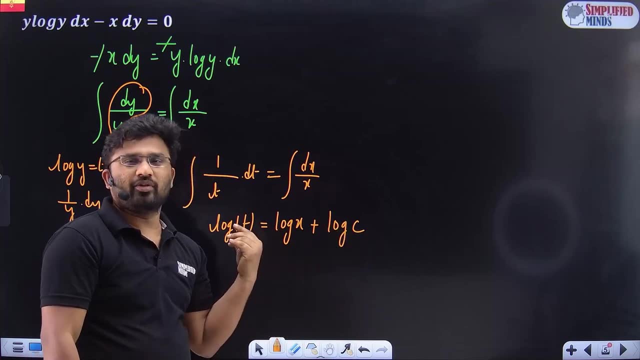 So if you ask like this, your log, you can you have to find anti-log of c, But for that you will still get the answer. But log c. everywhere there is log log. take log c Here. 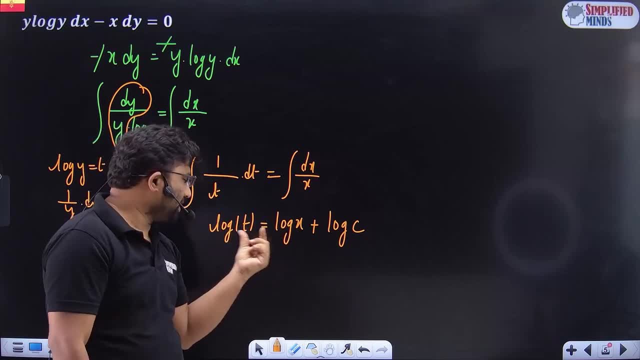 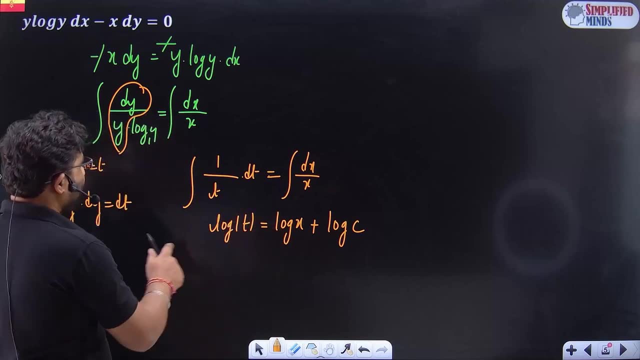 you have sign of x, sign of y here also. take sign c Here, e power x, e, power y, e, power y, e, power x. here also sign of y. Now, what can be done Now? log t. 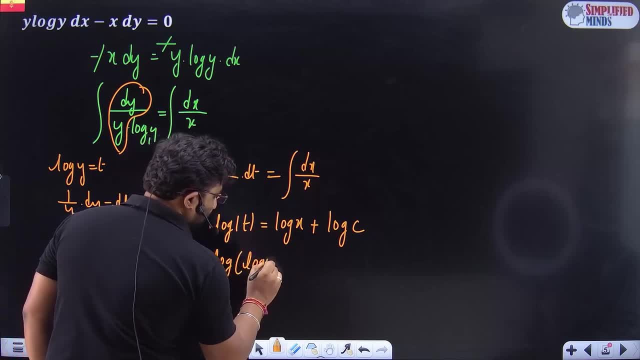 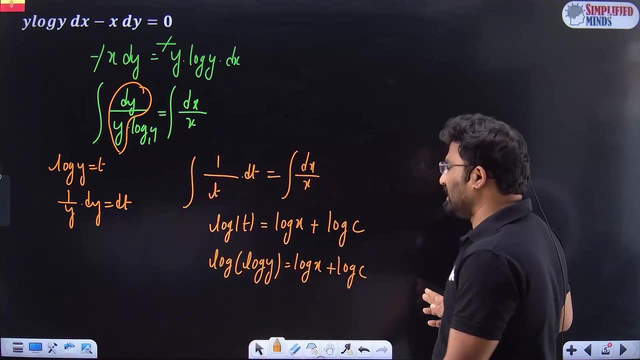 what is my t actually? Basically log y. So I do log of log y is equal to log x plus log c. So since everywhere there is log, I will easily cancel the log. But I don't cancel it. 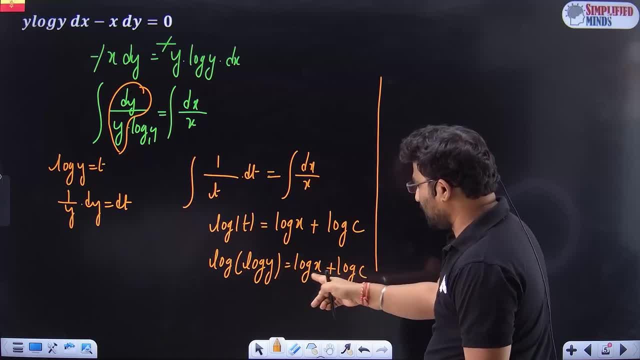 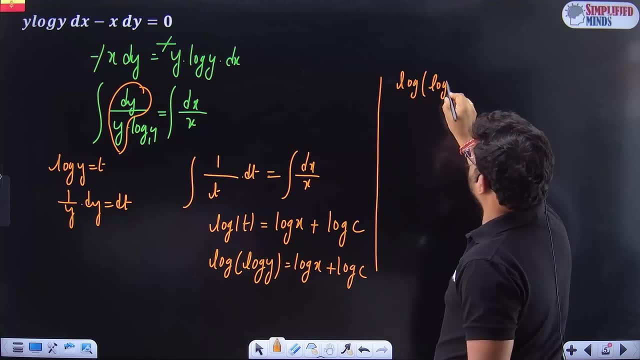 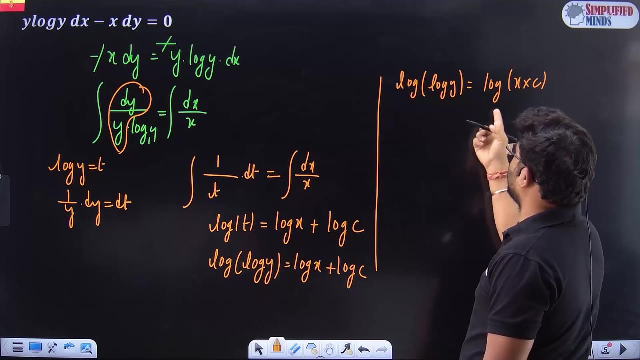 So I have to simplify here. So what to do? Log of log y. what is this? Log m plus log n, log m into n. log of log, log of log y equal to log m into x, into c, and that means so we can say inside cancel and tell about now. 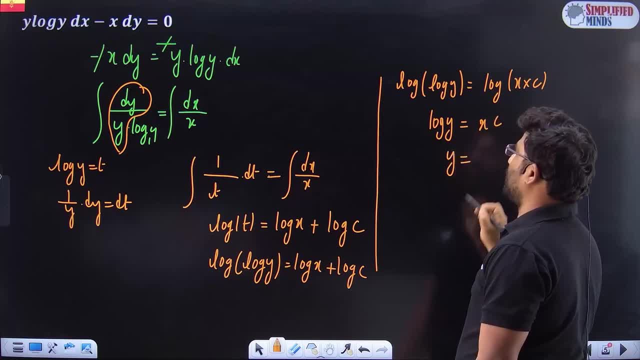 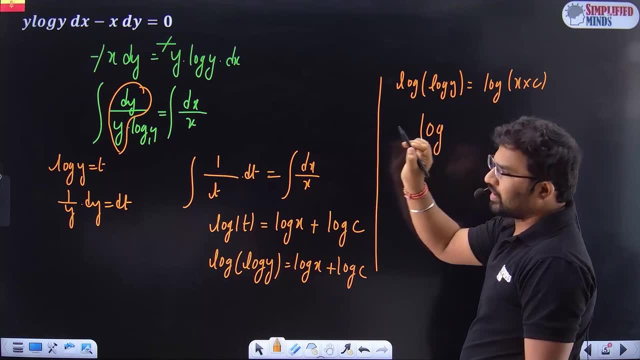 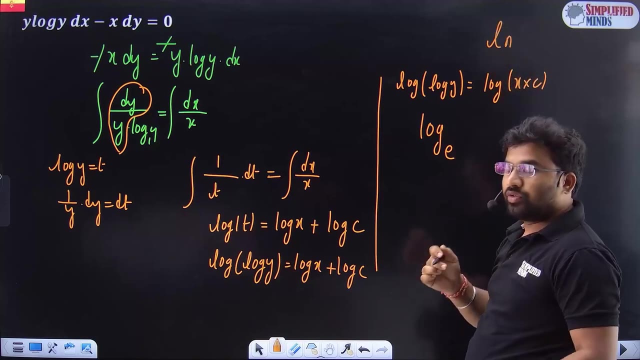 log y is equal to x into c, so y is equal to n markiga in particular, log log y is equal to the log see by default in any intervention. by default ever tagliero by default in fact. now ellen and burdett always see in one of the other real life problems early lna natural logs use. 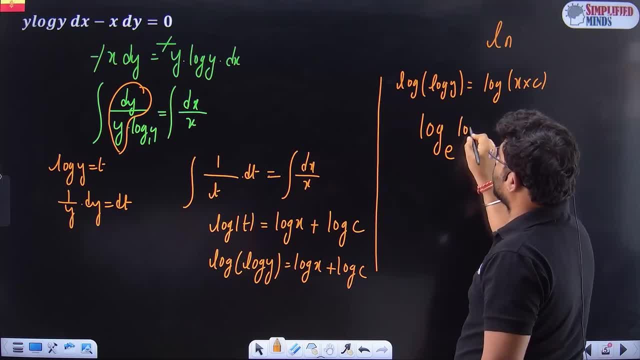 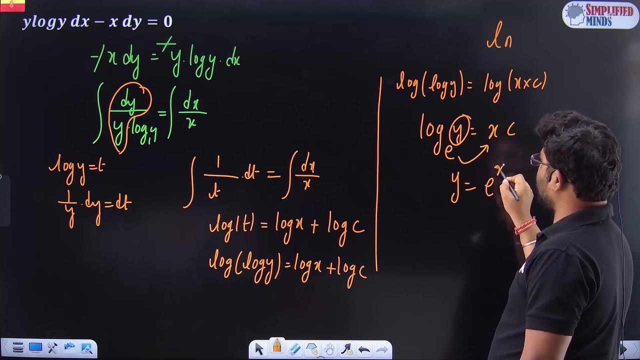 marty v or data by default here there. so it is log of y equal to log log here to cancel again inside value: log is equal to x into c either i want y, so y is equal to e negative e power xc and the answer is either about one will not have the logs in the corner. 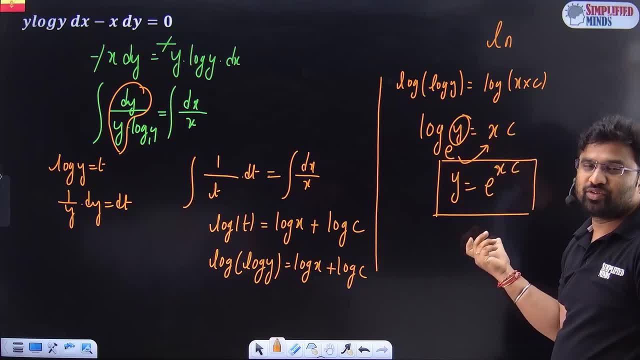 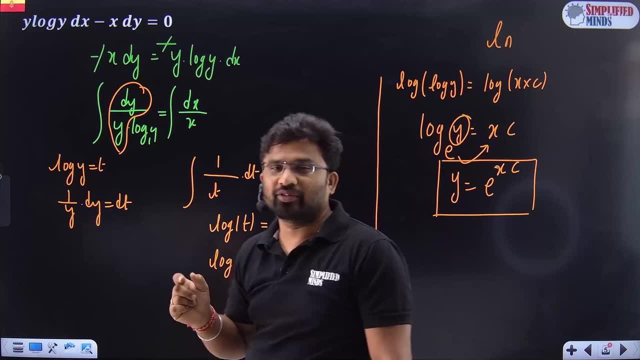 you. i think you won't be able to get so simple answer. y is equal to e, power, xc. and well, that's the. anyway, you can still take the answer. i think a boundary condition question could talk about that. and then our values: particular type, particular solution find. 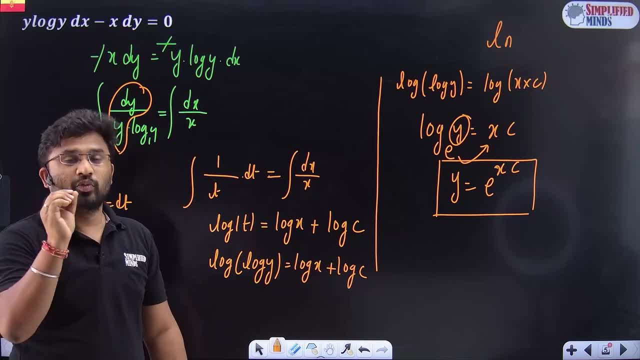 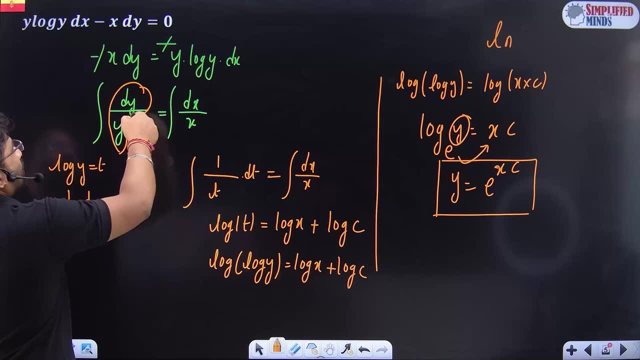 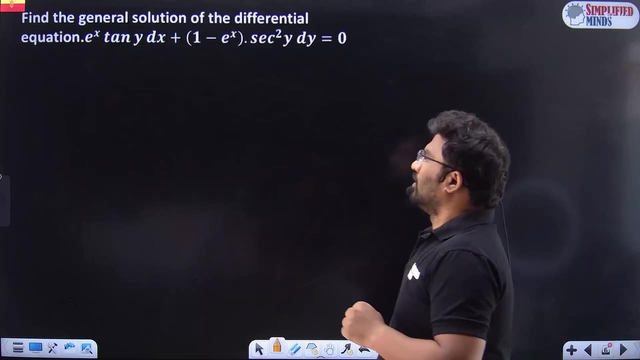 what i call now. i could try values, now that's directly again, so variable, separable and the variables are separate money, integrate, my way go. integrate model. you may get some additional type of, you should know proper integration, like substitution method, all the methods you could get right next to e, power, x and again. anyway, try maria. so you have to try, anyway, try. 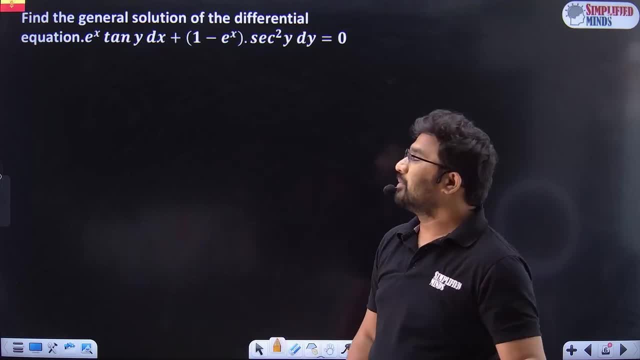 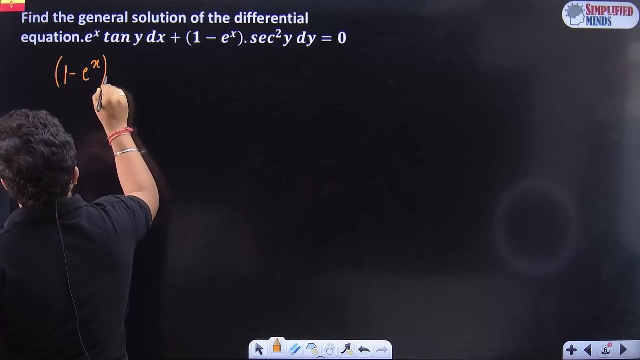 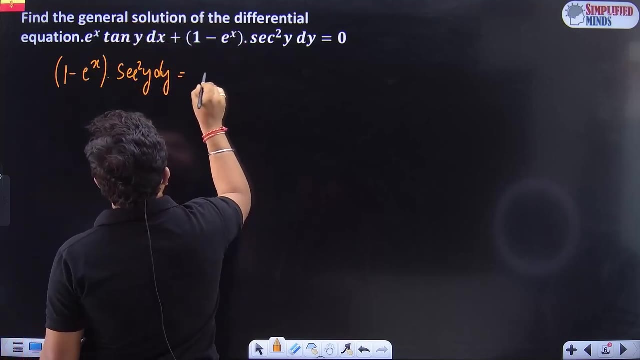 model. if you do not pause money, try yourself. take one thing now: one minus e power x into second square y, equal d y. so one minus e power x, second square y, d y. yeah, if you later that any, then you can shift murder any minus e power x and y into d x. 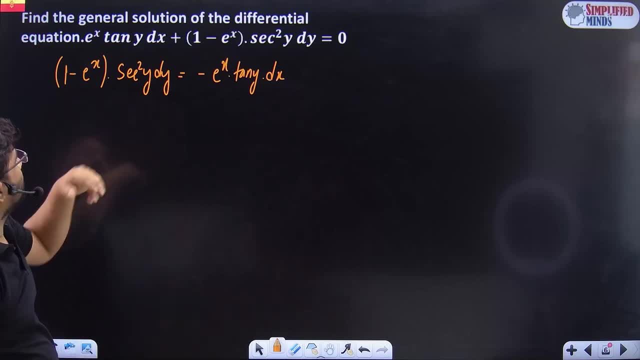 if one by e power x, second square, y d y equal to minus e power x, into tan y, into d x. now in monarchy we have to shift. y is one side, tan y could idea dx, e4x, academy, tan y, we can bring it this side. see tan y differentiation, second square: okay, i mean one minus e power x. now we have to. 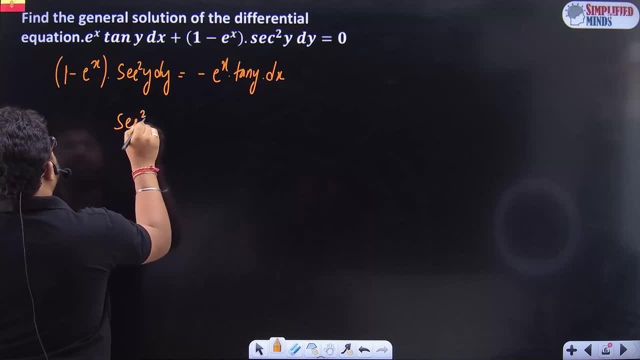 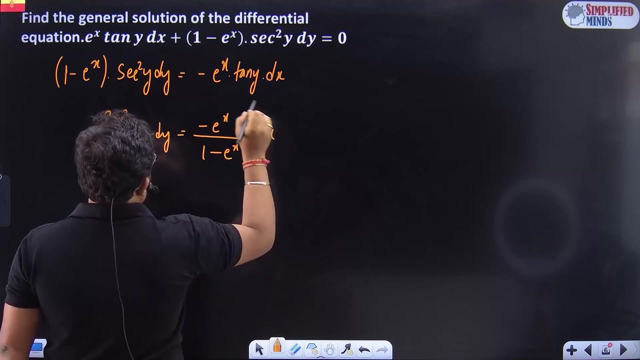 bring it this side. see now the answer again. second: square y, d, y divided by you can square y divided by tan y here d y here minus e power x divided by one minus e power x, one minus e power x into d x here. so yeah, name, name and lectures, node is a proper integration. yeah, what is the answer for? 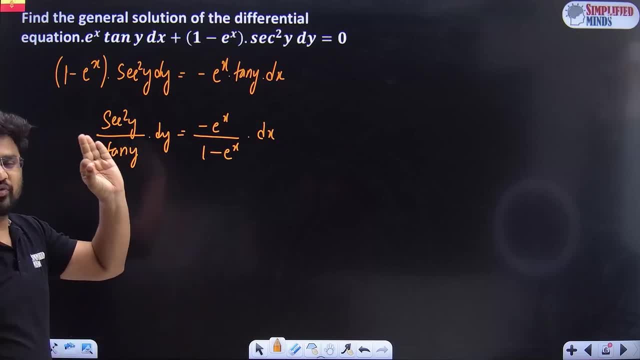 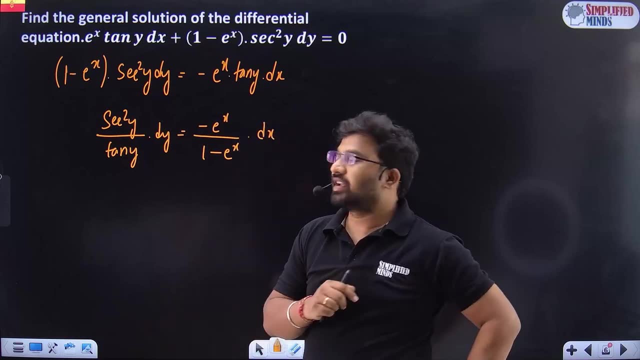 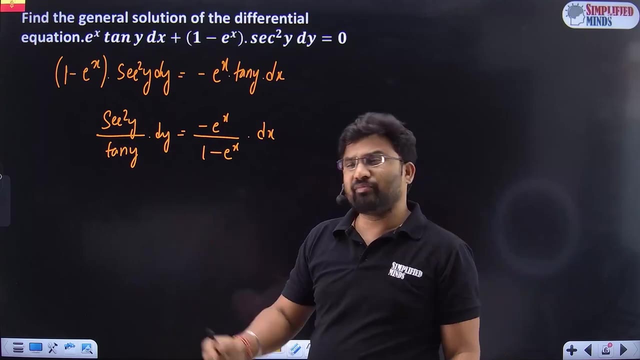 this. so it is in the form of f dash of x by f of x, f dash of x, and then you know, f dash of x by f of x. i mean what i kept dash of x until then. see denominator differentiate by numerator. so what's answer for this log, f of x plus c, and at the answer very, both in example, then you algae. 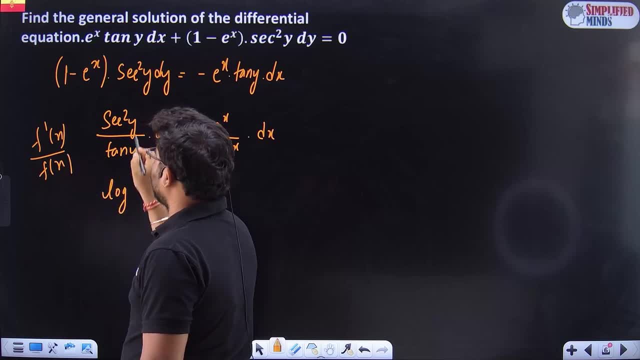 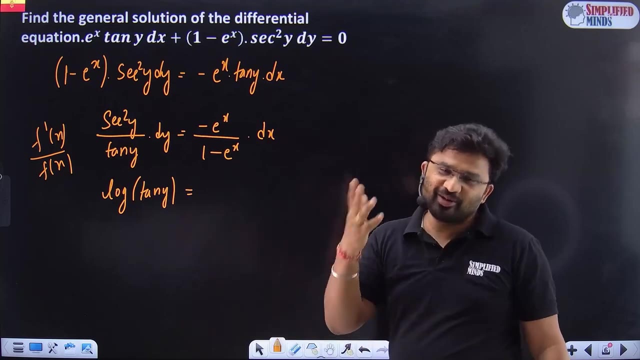 f, dash of x divided by f of x, differential. So our answer is: log of and y. What is the answer for this? Differentiate this one, differentiation 0, e to the power x. whatever we do, e to the power x will come, but minus is obviously. 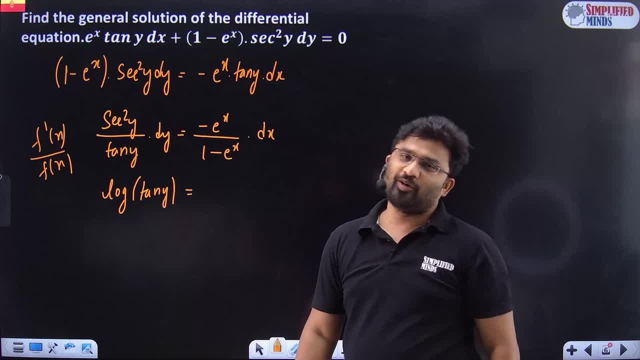 minus will come minus into e to the power, x. So it is also in the form of f dash of x by f of x. So what is the answer for this? Again, this also log of 1 minus e to the power. 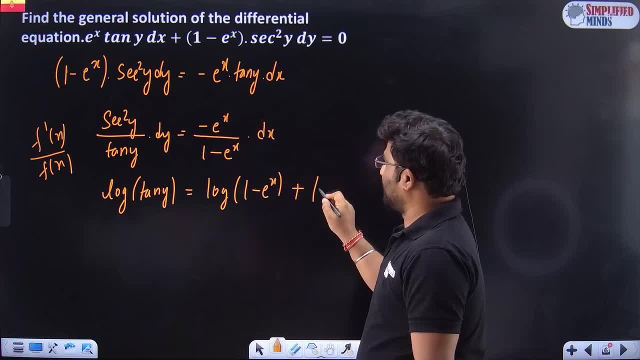 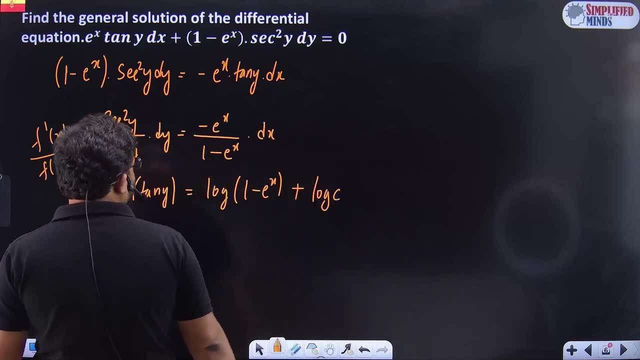 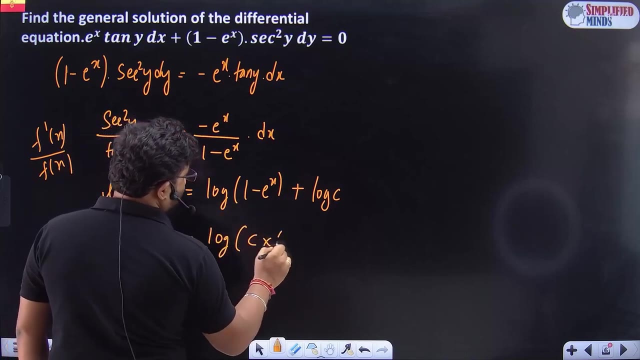 x. So what do you think of c? You think of log c, Log c. everything is uniform. it is not log log, Do you understand? So what is the answer for this? So you are going to get the answer is basically log of log m plus log n, c into 1 minus e to the power. 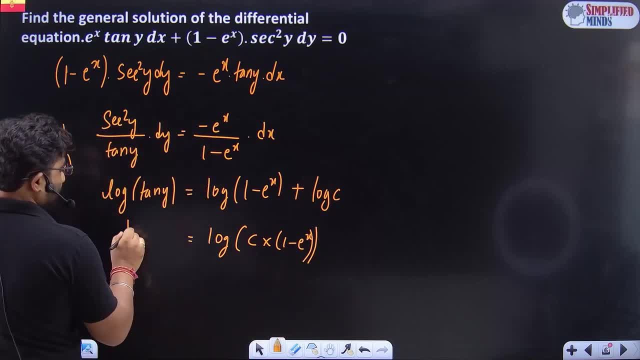 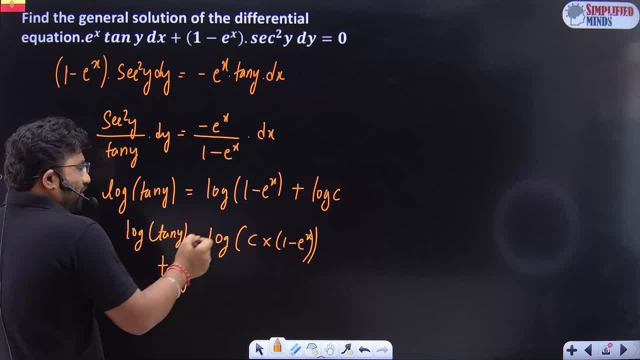 here it's not log in to cancel model, okay. so we should never say log log cancel. hello mccleary, sorry, you're looking at log. look at this log log cancel. and then it's not like exactly when one function is equal to other function if function e, function equated by controller, other the variables equal in back, other the. 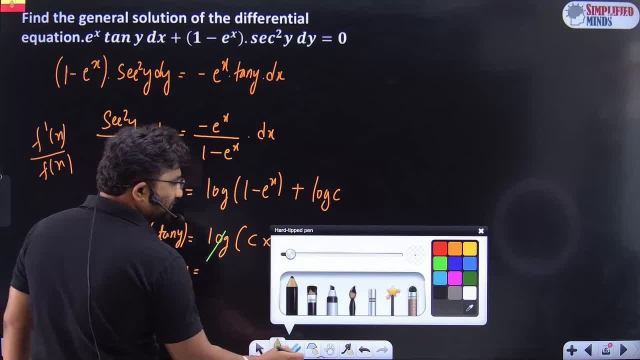 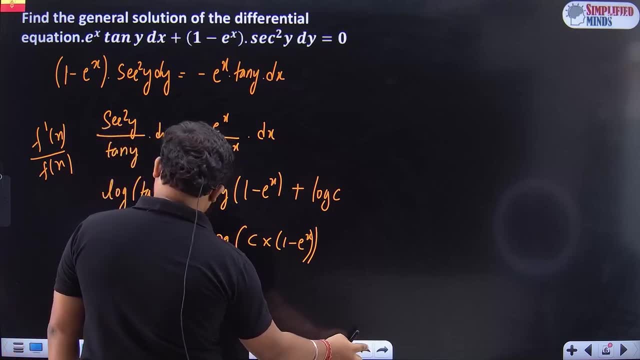 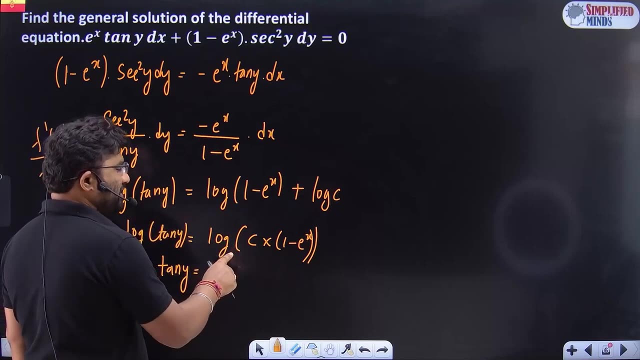 inside variables. so tan y is equal to. tan y is equal to: uh sorry, if you're arranging this, i'll do it myself. kids don't watch full video. they won't watch full video. then suddenly sir has cancelled it. they will also cancel it. because of that. tan y is equal to c into. 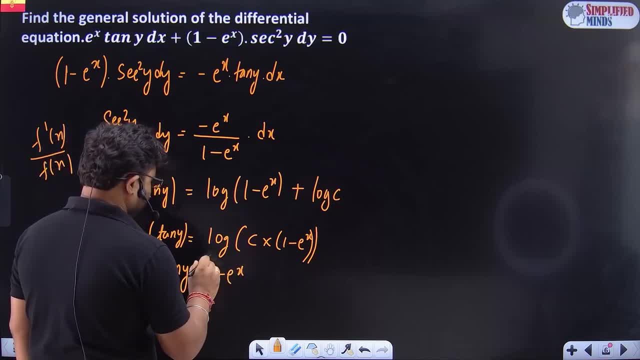 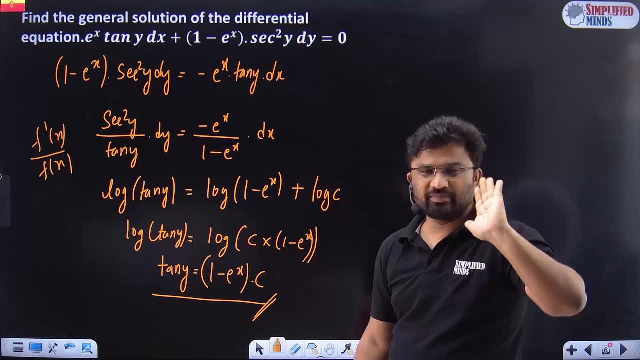 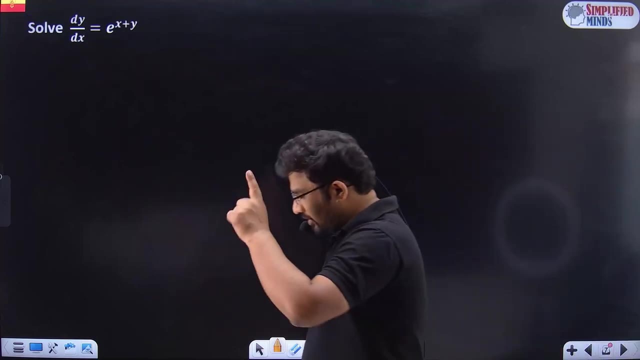 1 into e power minus x or 1 minus e power, x into c and then answer. it's a simple answer, right? so basically, kids, variable, separable, easy, easiest method. but your integration is good, because integration is good, this method is very easy. let's go for next question: video password. 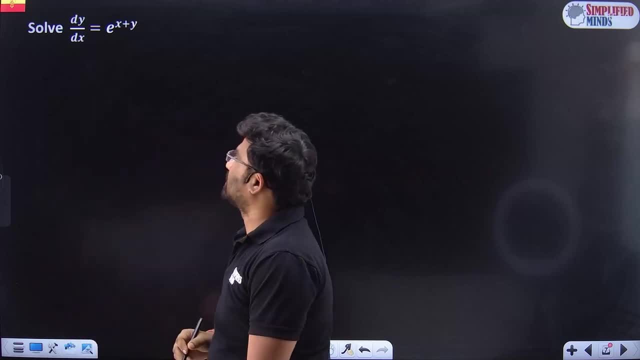 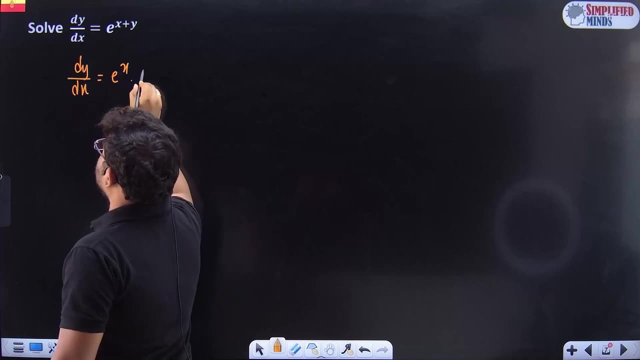 you try it. okay. first dy by dx into e power x plus y. yeah, so what can i do? dy by dx is like this: so e power x is e power x into e power y, and then i will write. so i will write dy by e power y. 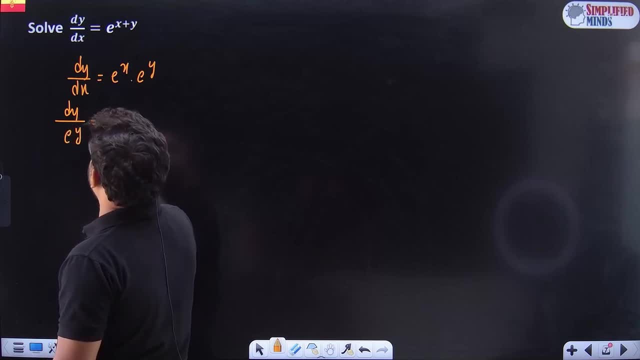 e power y, okay, and then e power x into. i will write dx. so if i want, i can write this as e power 1 by e power y and then e power minus y. it can be written if you do. well, now the power with the reciprocal here. 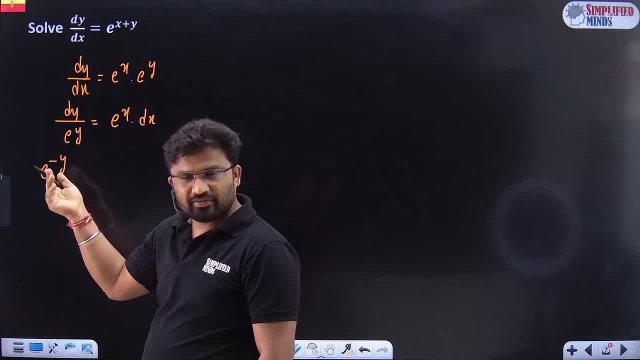 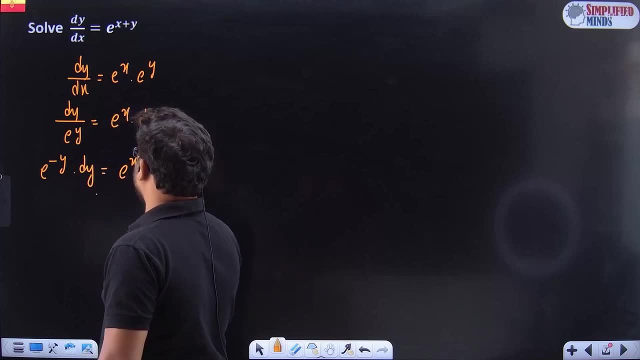 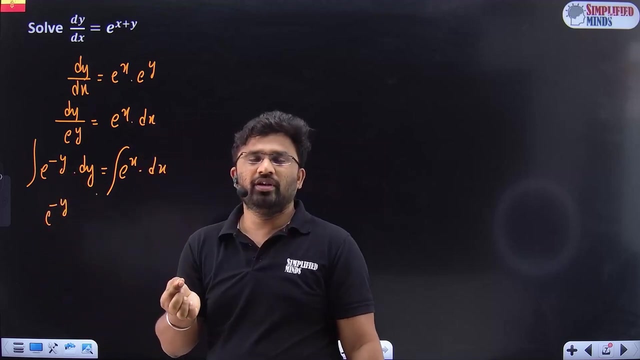 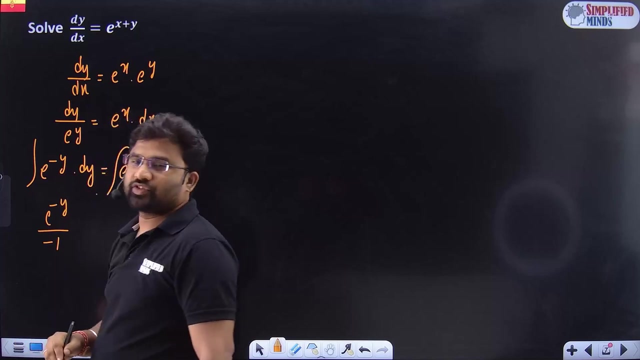 positive. power will change. symbol of the power: negative is positive, it will be positive, it negative. integrate and integrate e power has. this might be the integration c's or y's plus two minus two, x plus three and the other in the differentiate Marty. divide Marty and tell either in PDA the minus by differentiation, when the minus one. 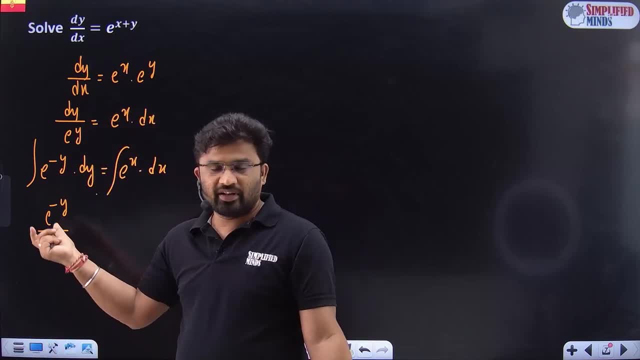 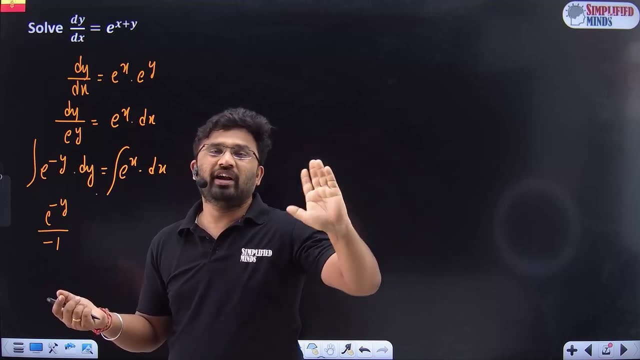 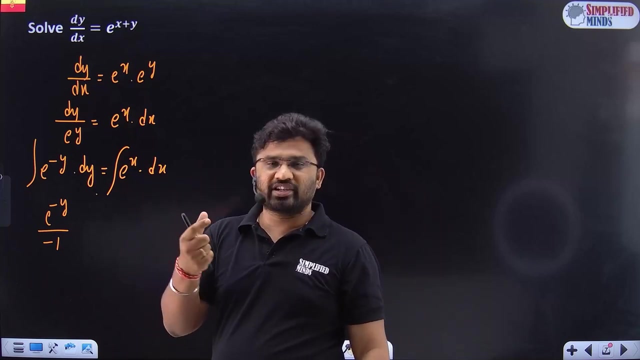 over time and the differentiate mother and divide, mother minus divide more like: oh so differentiationally multiply more TV integrationally divide. Marty, we did an integration to market a helicopter in the Adam or lecture cell and Haley, Vinnie, 2x plus 3, you sign 2x 1, 2, sign 2x the integration, what I can. 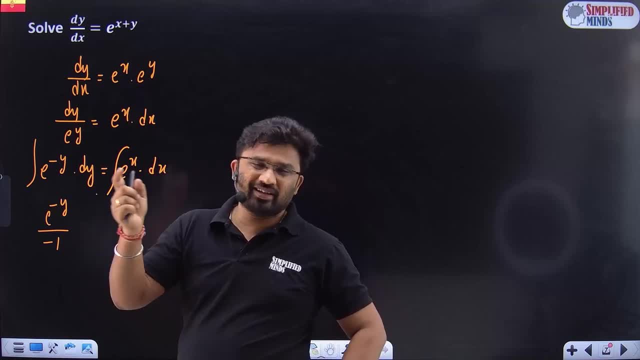 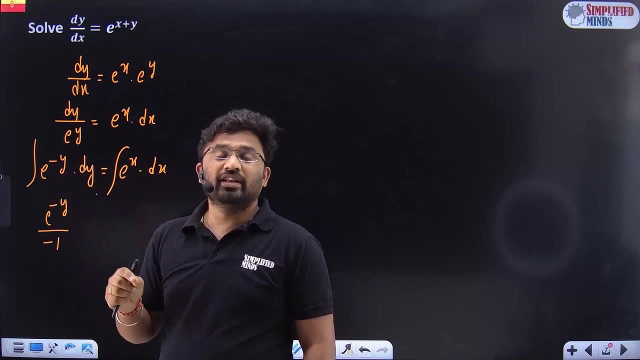 do. actually I can actually made it 2x nutty and to make them attend to DX equal DT in my record not required, it was actually made it minus my nutty and to come back, oh okay, then we power T the e, power minus y Lula, and I'm a trap. 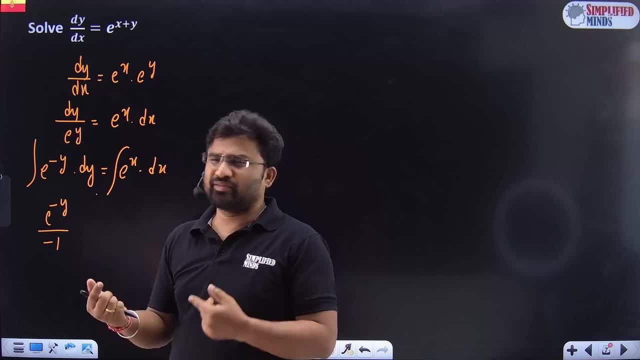 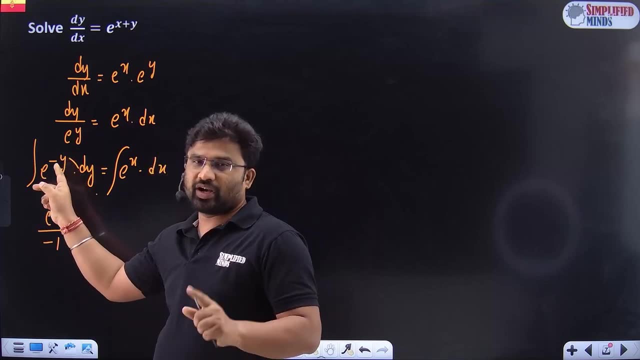 formula, but the matter T, and to make them, at the minus device, equal to minus DT birth. and what a negative. a charitable not required and even more echo, a poor way, a poor wire. the minus y, the differentiation, why differentiation? one year of the minus one, minus one, and divide, Marty, integration and divide. 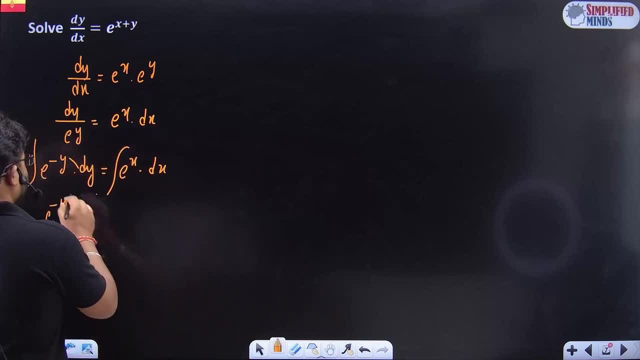 Marty, we differentiationally multiply mother chain to Lama. yeah, he'll, you do idea, but do anything. integrate, Marty, and already e power X plus C and the paratha. we'll now see if you, if you want, you can take this also as e power C and we're the only uniform element in mana: e power C and the one next to minus a. 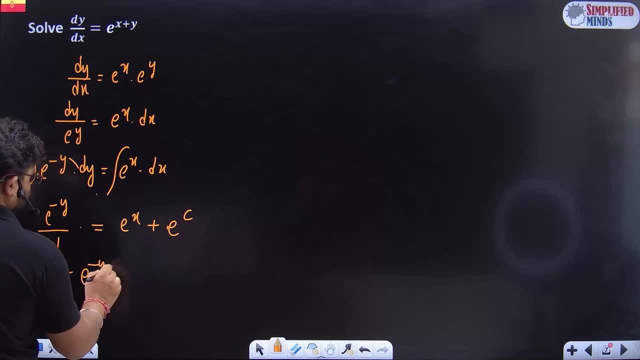 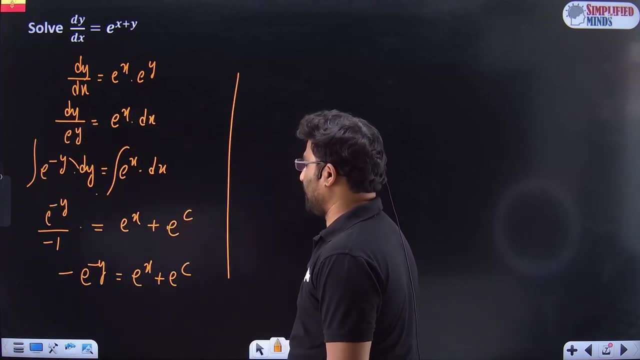 minus little one and minus e power, minus y equal to e power X plus e power C and Tony Norena in birth number two. so if I shift, if I shift the d4x, that side. so minus minus e power, minus y, minus e power X. 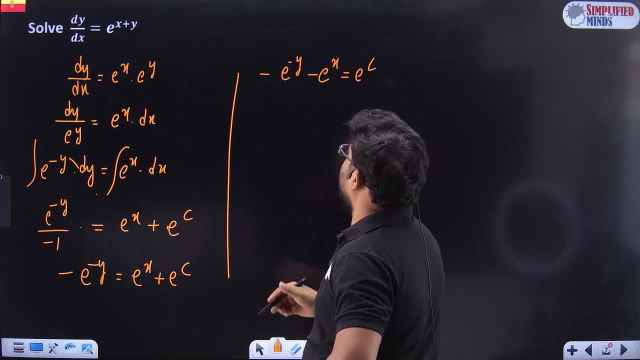 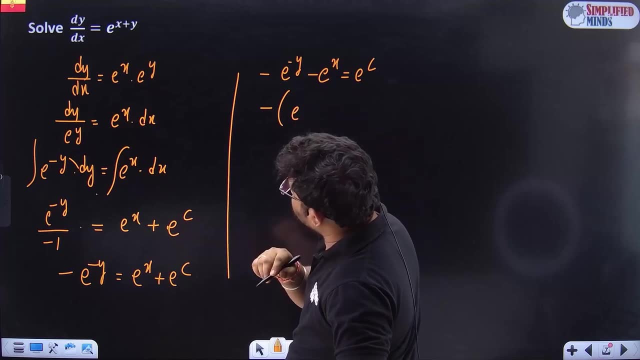 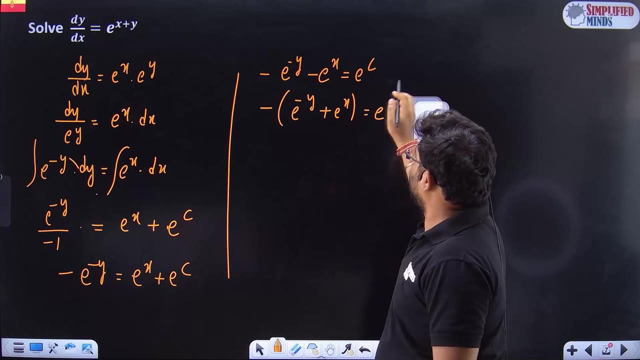 equal to e power C and the birth either, and the negative common town, right, my negative common town to e power minus y. okay, e power minus y plus e power X is equal to e power C, e power C and Tomada, or we don't have to cap the formula. no, a power m plus a formula. there's no point. 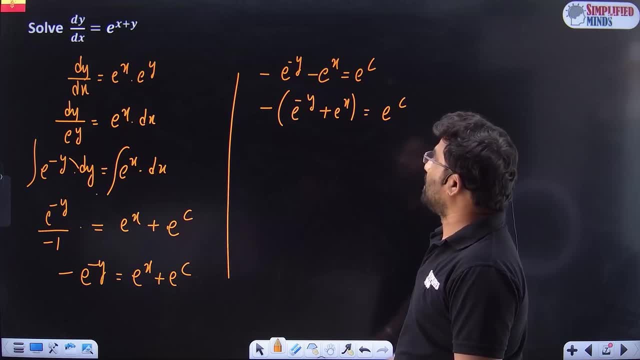 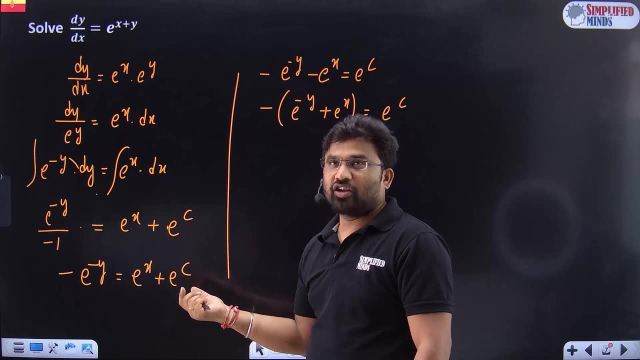 of taking e power C, because in the camera don't really multiplication of the, the road, one, the way, the enemy. hence e power y into E power X, E the right we have taken, eat power series, either have a new material, quit mara, get so fritipayah exponents for equate mother, like it. so he leaves in, you know he. 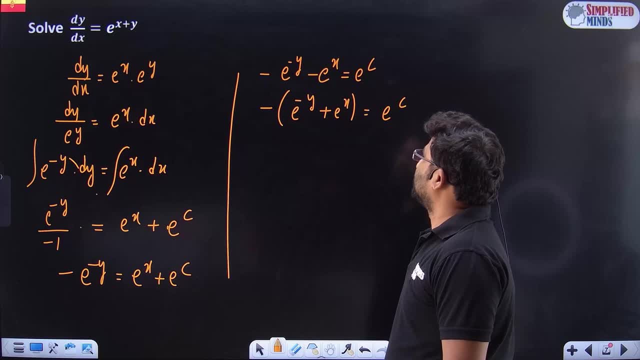 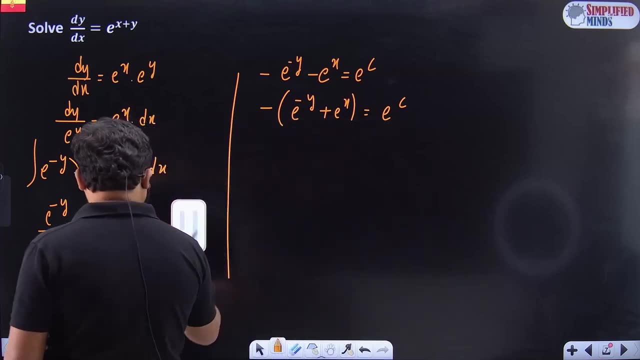 personally took on the a: no mother birth. I'll actually simplify, Marlora, you know. okay, not a problem. so you'll get a power c, which means that you have to combine the e. power c is not necessary. We can take directly c only Because if we take it, we have to simplify. 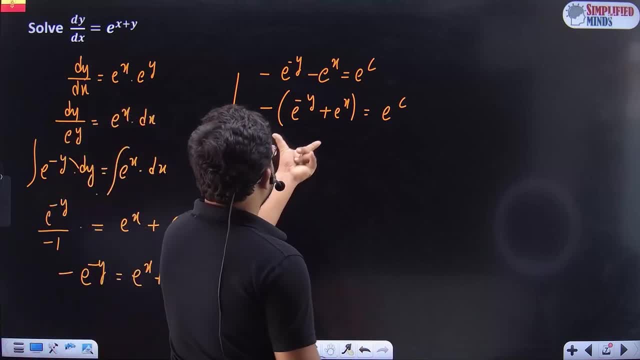 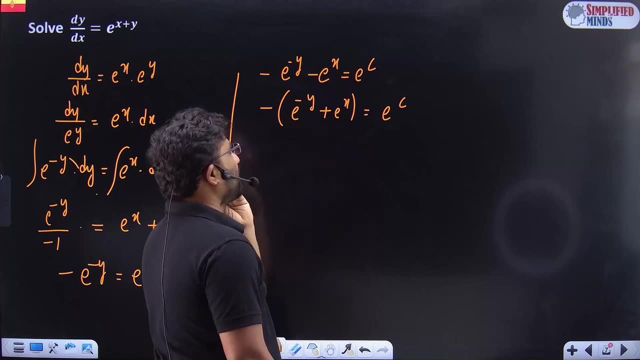 it If we take it, we have to simplify it. We have to simplify it. See what we have to do with this. You know, we can do it, even if we cancel it, But we cannot do it. We can do it only if we have multiplication. There is addition. It is not possible, So we have 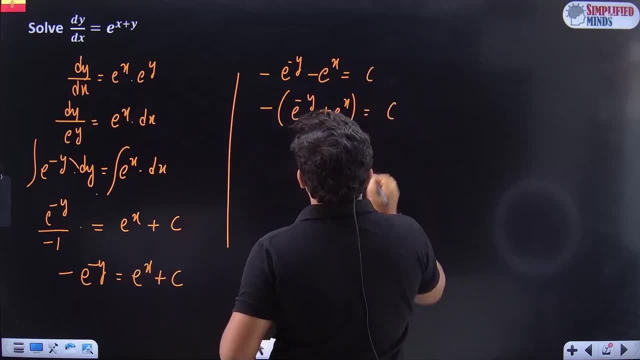 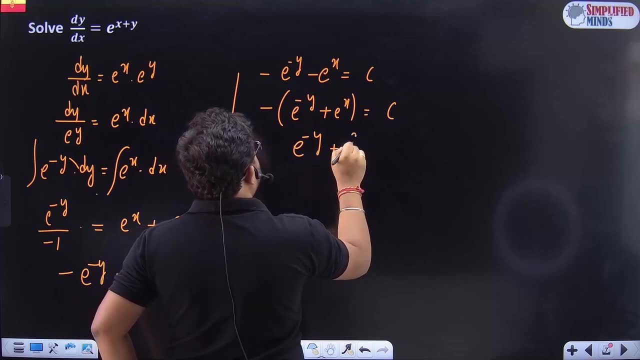 to take c. That is it, What is there? We have to take c. So this is the final answer. Again, if you do not want to keep this negative, shift that side. So we have e power minus y plus e power. x is equal to minus c. Instead of minus c, we have to take another variable. 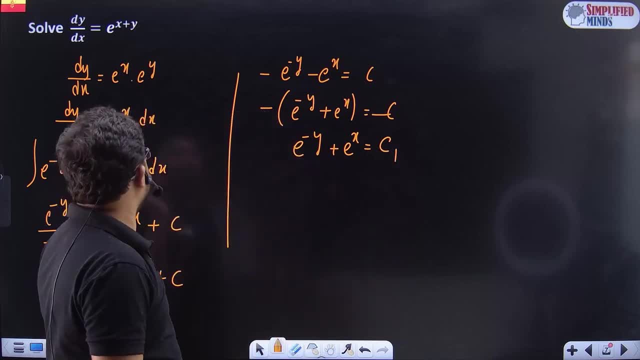 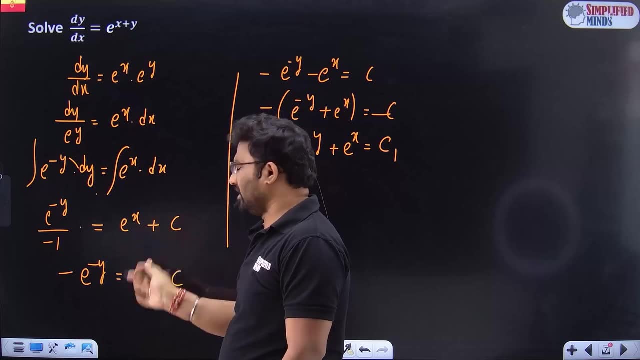 c1.. We can change the constant. Next, dy by dx. you have to get dy by y this side, and e power. x is minus y. Integrate it. That is it. It is not easy. This is how it is The. 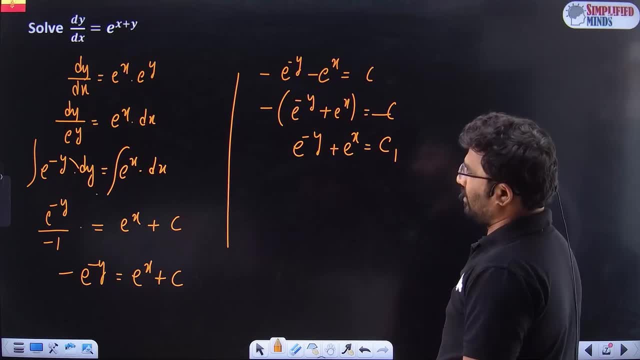 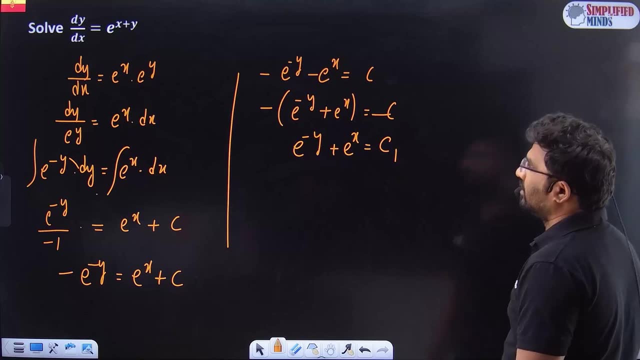 answer is: e power minus y plus e power x must be equal to zero. dy by e power y dx into e power y. Next, let us go for the next question. Next, it is a simple word problem. It is not a very 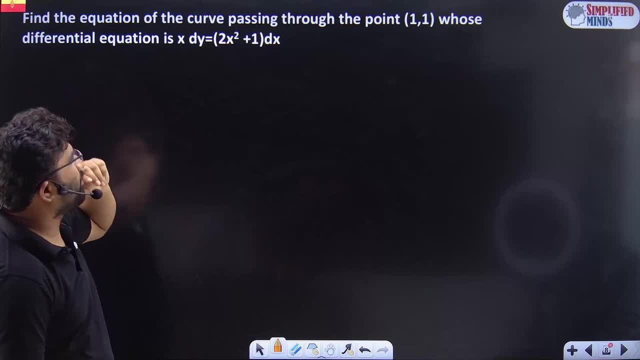 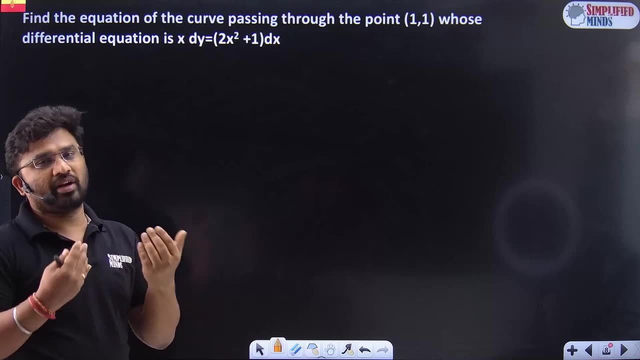 difficult question? Simple, See: find the equation of a curve passing through the point 1 comma 1, whose differential equation is given. And then what we have to find? We have to find the equation of a curve, That is, the curve equation is usually y is equal to f. 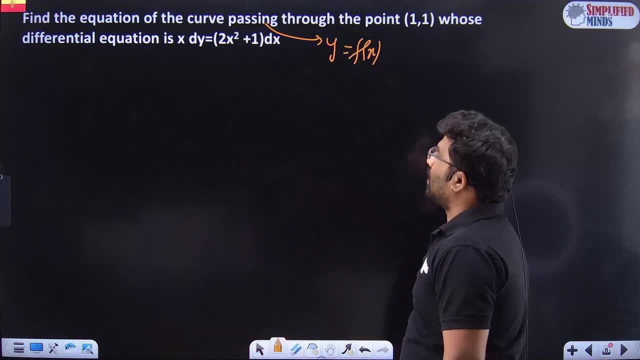 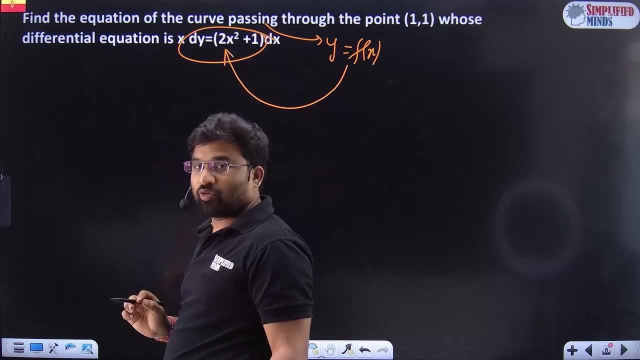 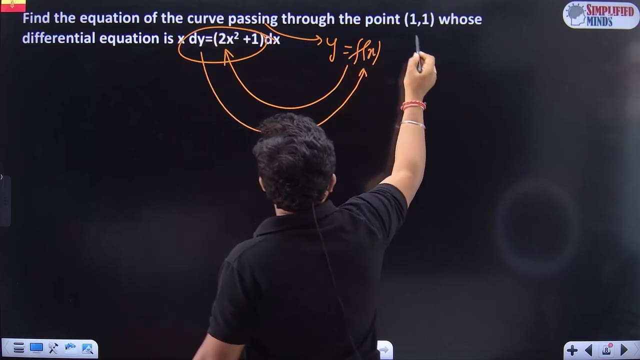 of x, So y is equal to f of x, So y is equal to f of x. is the solution? We have to differentiate that and get this answer. But this is not the case. they have given a differentiated form. We have to find the solution for this and we will get it. The solution remains 1. 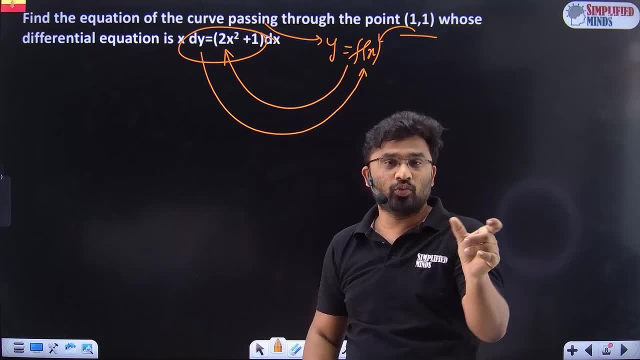 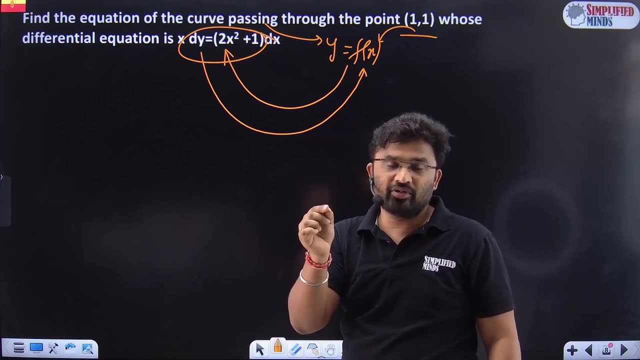 comma 1.. We have to find the c value after 1 comma 1.. I have tried in the previous lecture. You get a family of curves Now. it is not to say you cannot calculate c values. I told you last time in the lecture. For example, x square plus y square is equal to c. it is 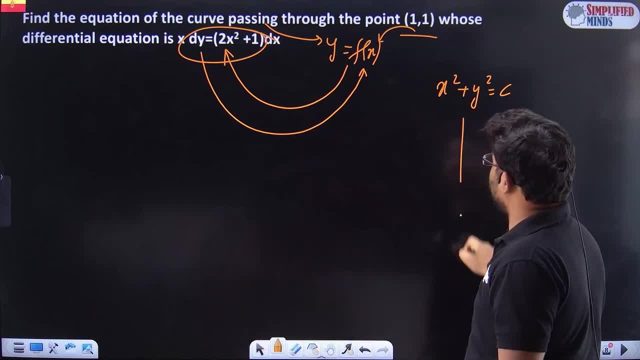 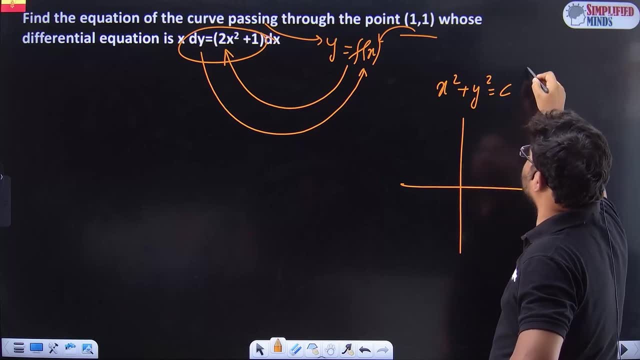 a family of circles. It will be not a diagram. It is a formula to calculate this. It is an actually forming differential equation in board exam in ncrt. but as per new ncrt they have removed that. it's okay. x square plus y square c, so you'll get a family of circles. 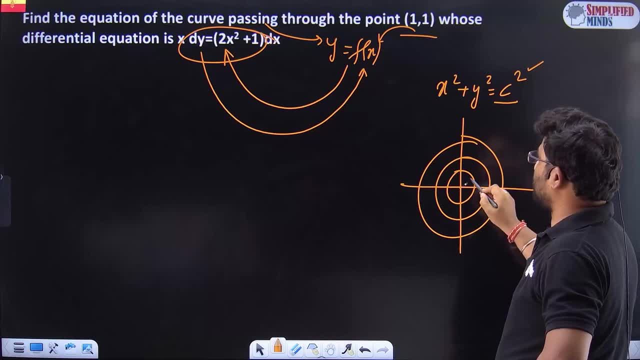 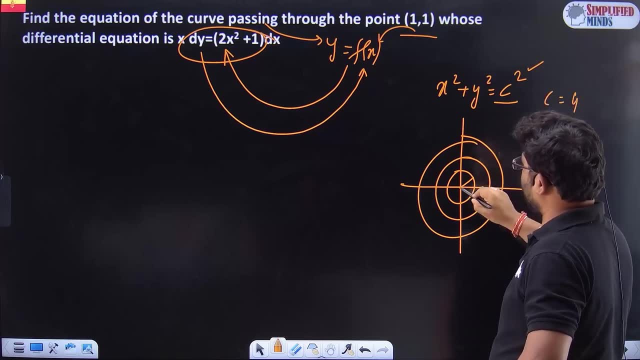 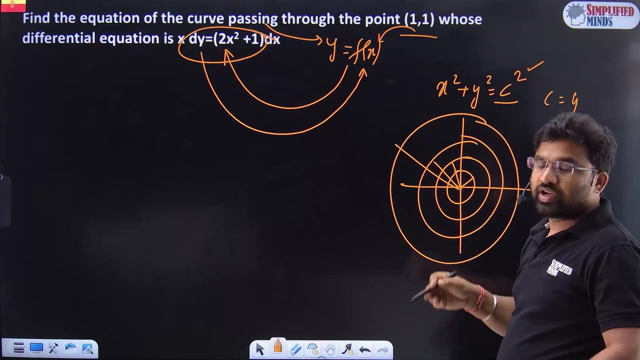 with different. as c changes you can see 2 on the radius 2, root 2- sorry, root 2, i mean root of this- and c, for example 4 and radius 4, the radius value change. but all the circles, what is common center is 0 comma 0. you'll get family of equation. that's why the constant. 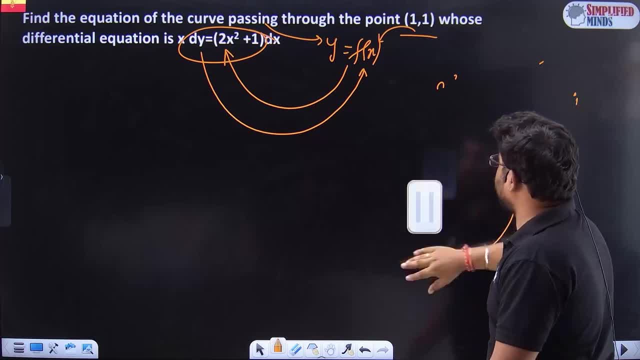 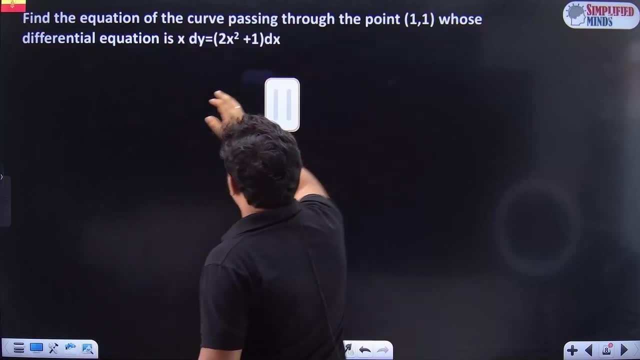 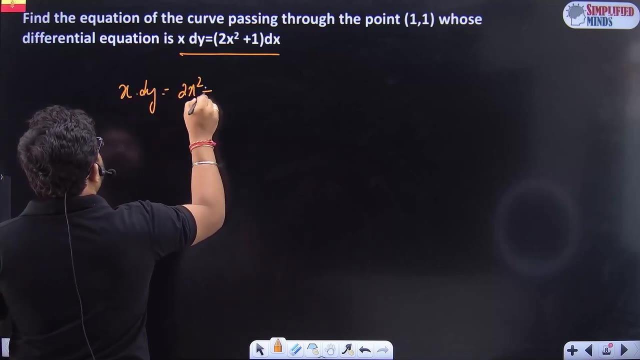 find model and the family of equation both outside. now you got nobody next to me. way more wickedly it again. it's very simple question. i mean, what i can get simple again if we just solution, find more casting anyway. so x into dy is equal to 2x square, that's 1 into dx. 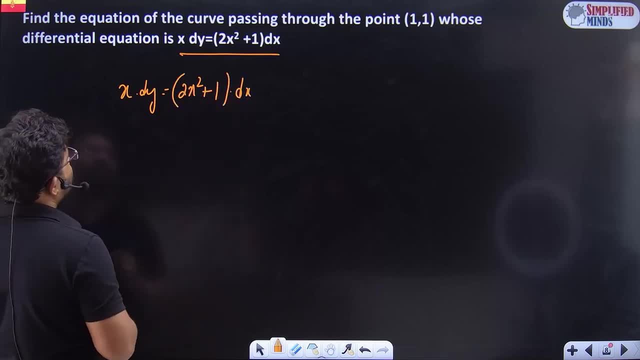 in what it now we got, oh divina, one. crush if money could be x now, and crush if money will do. you have a right there. ok, d? y is equal to 2x square plus 1 divided by x into dx. i'm a line model echo to integrate. 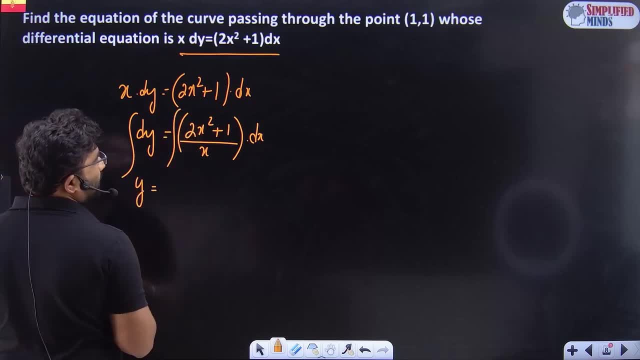 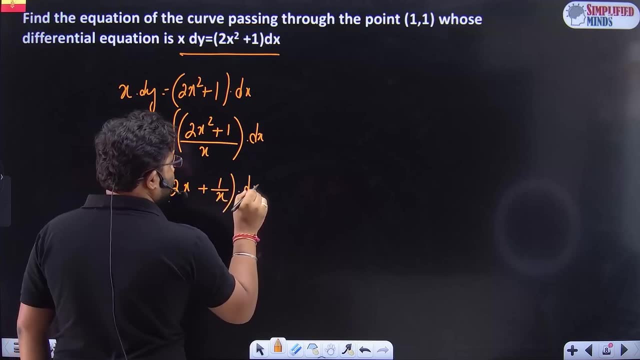 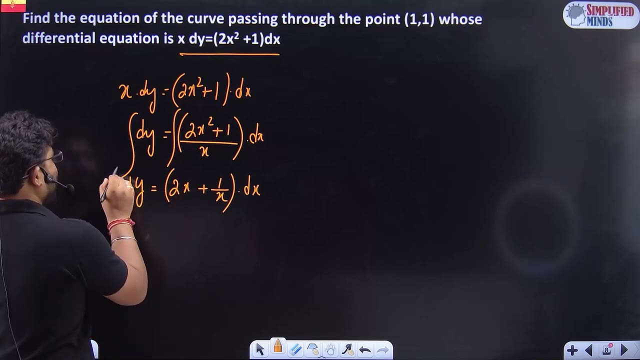 it. so d y integration. oh, why were at that 2x square by x in out there, 2x bar up there? you do 1 by x bar up there into the x. but i thought so when i integrate my lindy integrate model. okay, let's keep this d? y only. 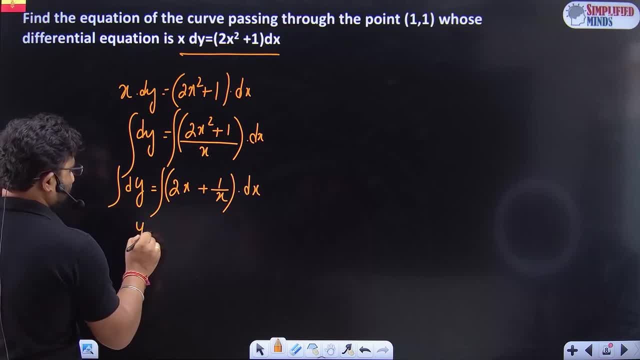 d, y and i put here: okay, okay, so d x, log x, mK. I do. you know, I don't know. okay, okay, do anything, but I'm gonna. marks might keep your short, and so that's the same whole thing. by the way, interesting, if you mean to keep you shirt by a ordinary 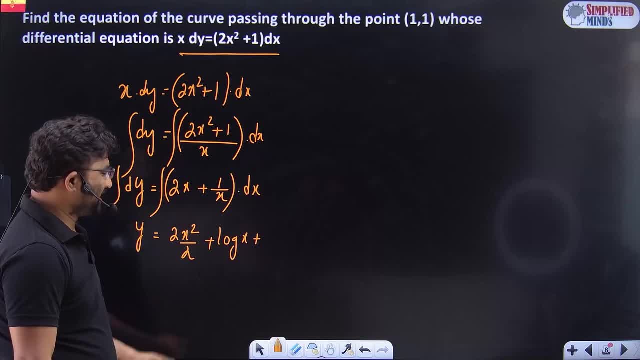 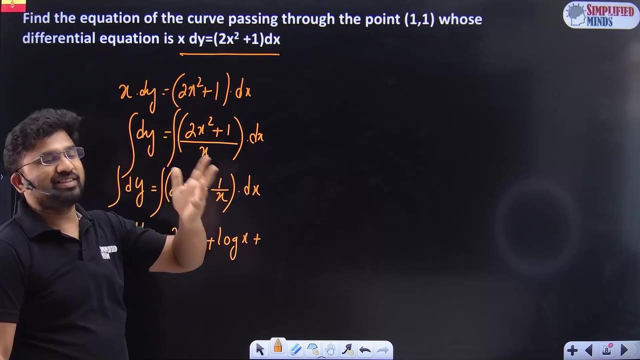 if you like. so in Tlux in a integration logics, integration logics or is interest of logics and number globally, and i'll second years like Charlie in and complete comedy formula: typo: integration of mobile X-Logic maybe, mister, intelligent-like, simple registration, opposite integration, user patients will become. it is. 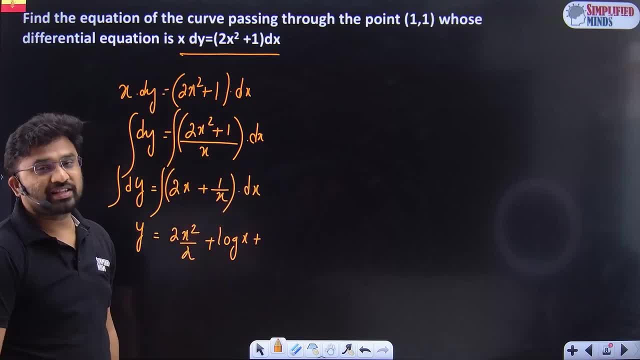 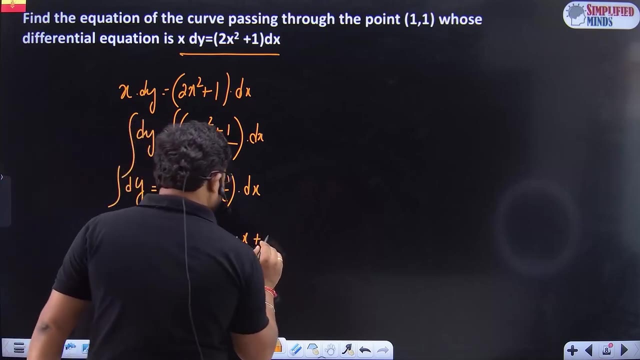 integration, no sir, and the integration of log X, 1, 2 X, log X minus X, X, log X minus X in my L murdering integration by parts, now one and the one. do only I late use money, modern NP dia and pretty London in bit come eco next plus C, the. 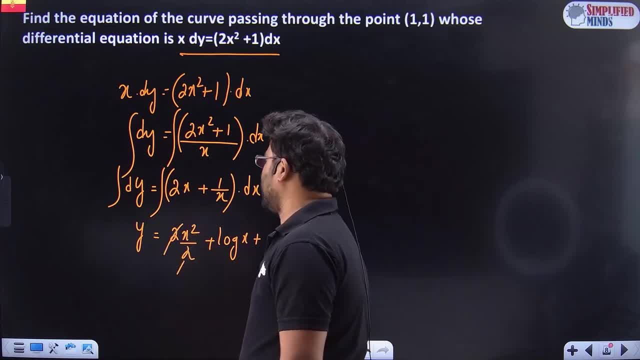 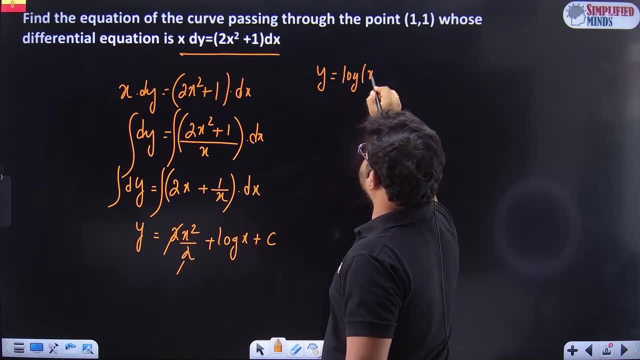 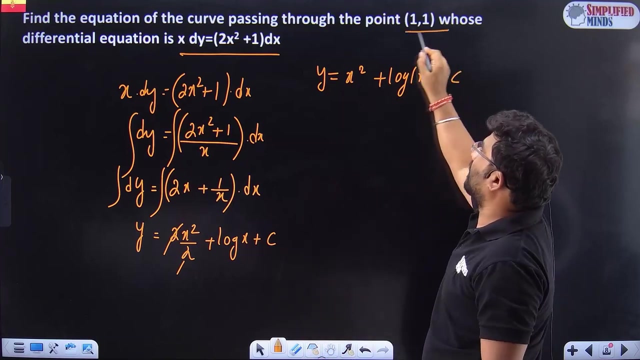 answer is what the law to? to cancel over to them. yeah, so y is equal to x square, y is equal to x square, log of log of x square plus no log a la x square by L was sorry. x square plus log expert plus C and the. really well, and think your point cut either and 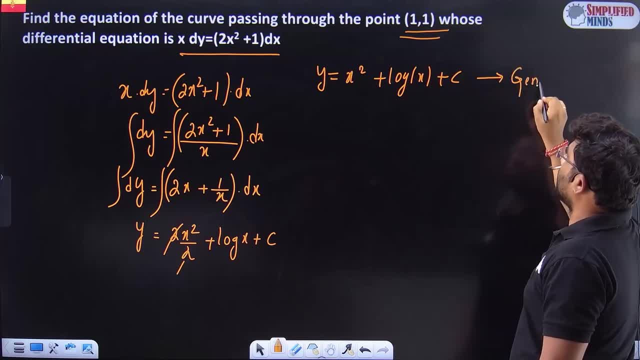 he'll only muck me last lecture, he'll do the general equation now generally question the correct TV. that will, I remember, go particulars, particular solution. or we can also call particular particular solution, the HTML particular, the particular value, see when the other value. are you to get a particular equation and they find what they're one. 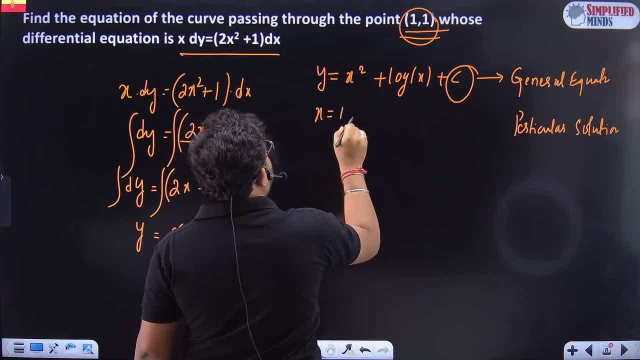 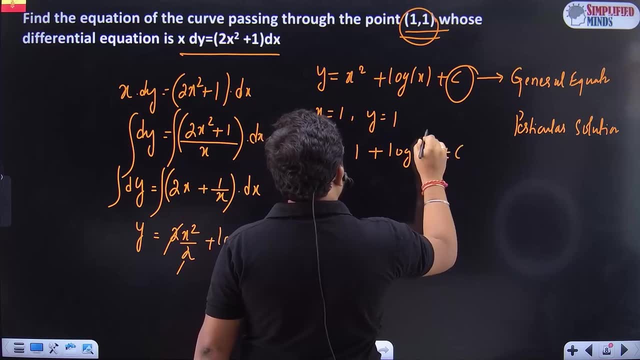 come on, substitute my naviga. so when X is equal to 1, Y is also 1, put 1 here, 1 here, log 1. so log 1 is anyway 0, 0, 0. I to 1 minus 1, 0 I to 0. equal to 0. equal to C. 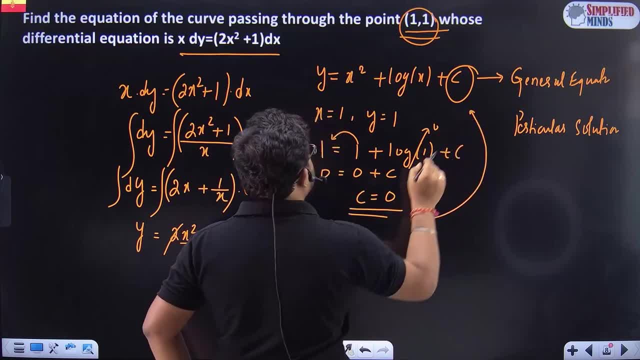 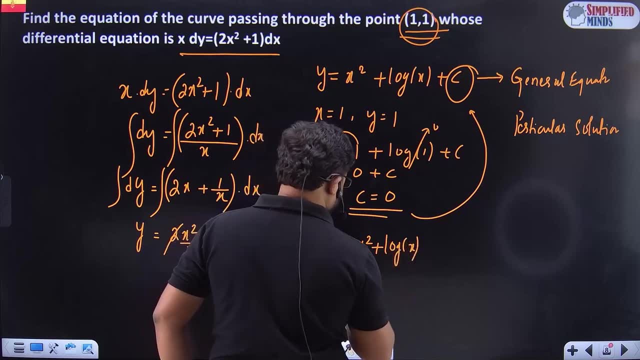 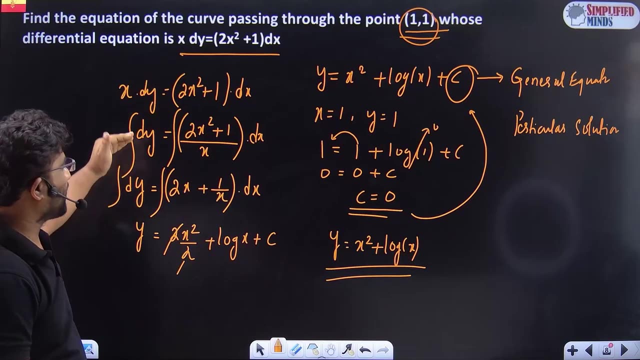 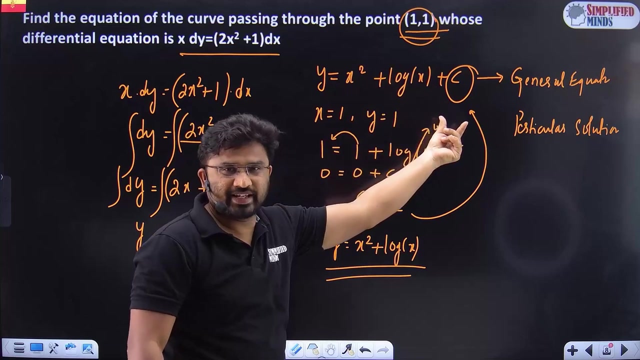 C must be equal to 0. is he rocker substitute accurately separate mother? and so the answer 1, 2 y is equal to x square plus log x. and but I simple again, we still find Monica, normally you try questions cut a normal integration, merica, defense, difference a question: are solving our 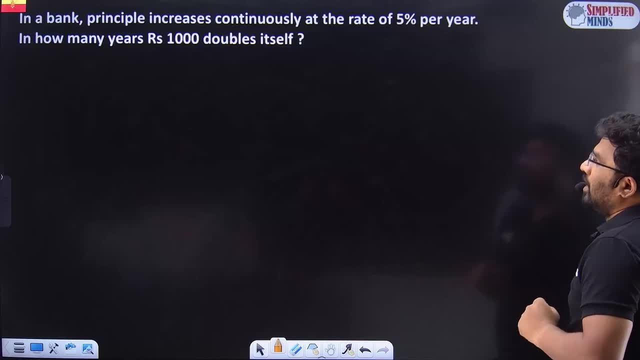 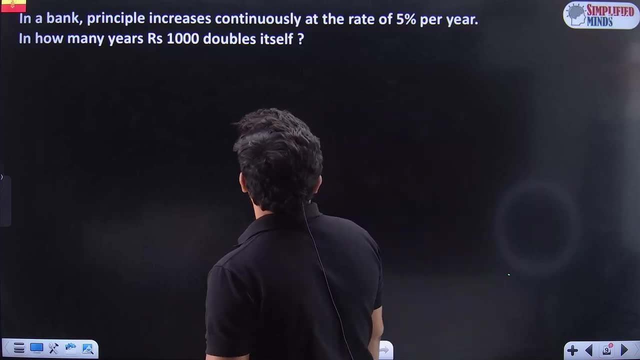 ok, next, next to next to in a bank. See, the question is given like this: In a bank, the principal increases continuously at a rate of 5% per year. How many years will it take 1000 rupees to double itself? 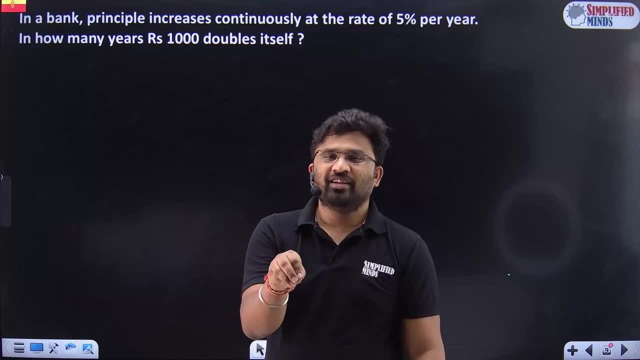 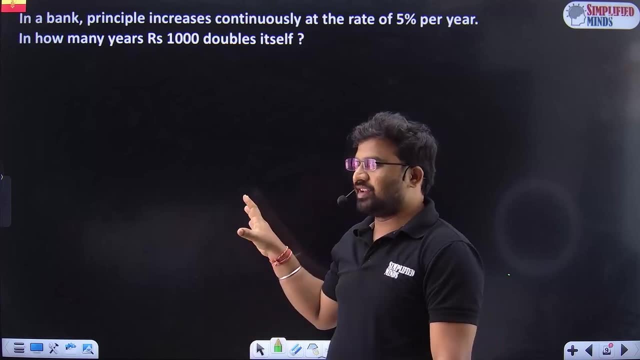 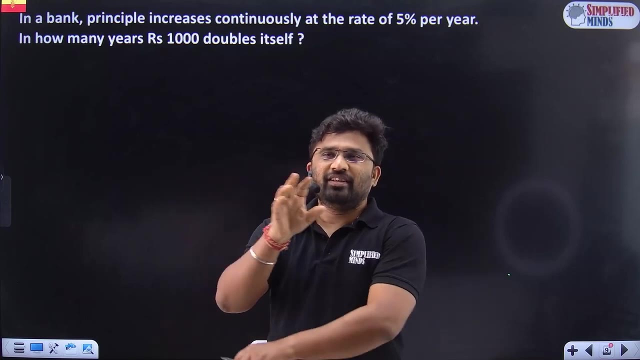 So you know, if you have a debt in the bank, your debt will increase. So how many years will it take to double? This is another thing that I will tell you as an out-of-topic topic. If you have a debt in the bank, no one has told us that there is something called as financial knowledge in the bank. 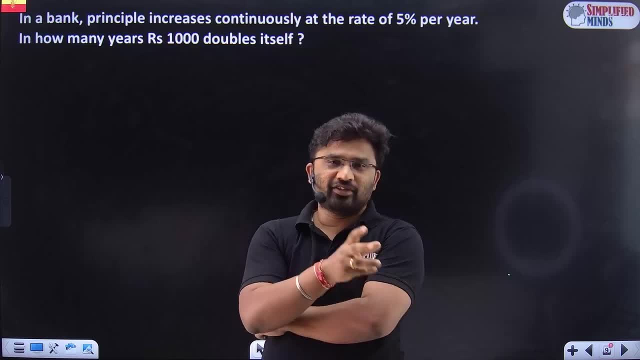 If we say that we have to go to school, we have to go to college. If you have a debt of 1000 rupees in the bank, you calculate and see how many years it will take. 5% Of course, in the bank. if you have a debt of 1000 rupees, you calculate and see how many years it will take 5%. 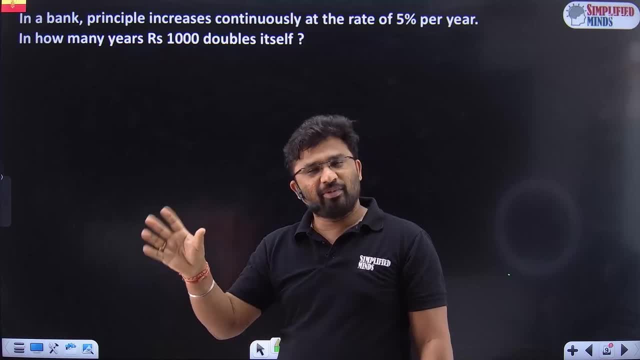 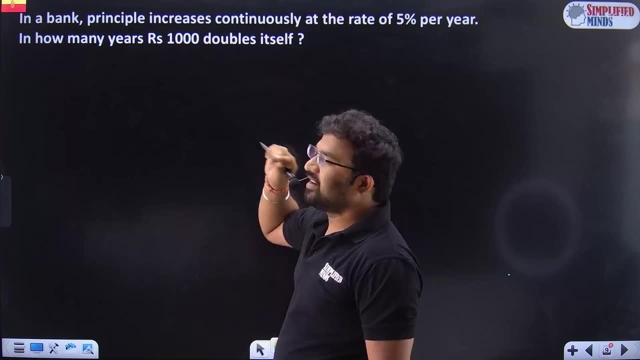 6%: 7., 8., 10., 11., 12., 15., 16., 17., 18., 19., 20., 21., 22., 23., 24. 25.. 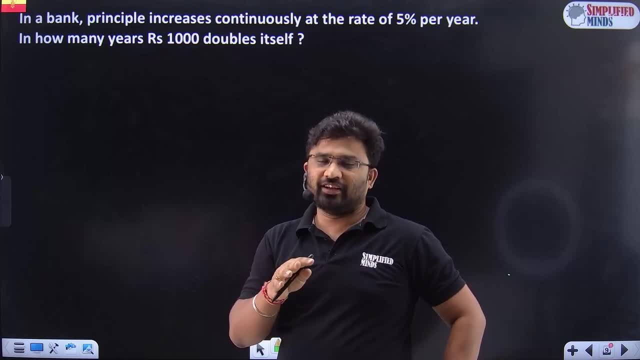 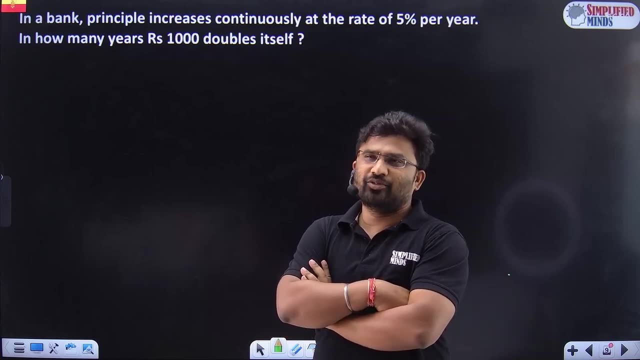 26., 25., 26., 27., 26., 27., 28., 28., 29., 29., 30. picture 33.. Instead of buying a car after 3 years, I used to buy a share of Tata Motors. 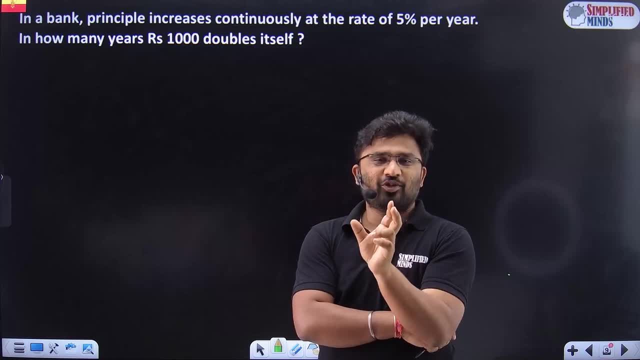 When I bought a stock, I used to have a minimum of Rs.1 crore and Rs.1.5 crore That means in 3 years. I used to have a stock price of Rs.100 or Rs.120.. Now the stock price is Rs.900. 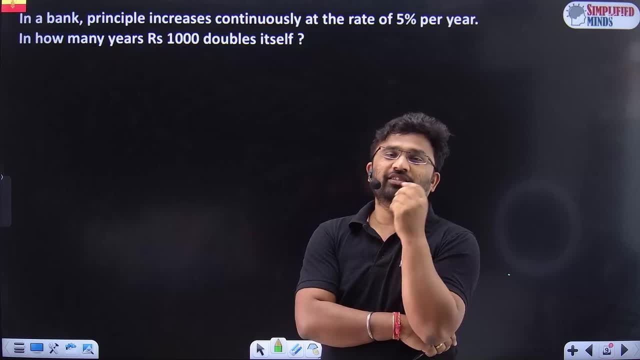 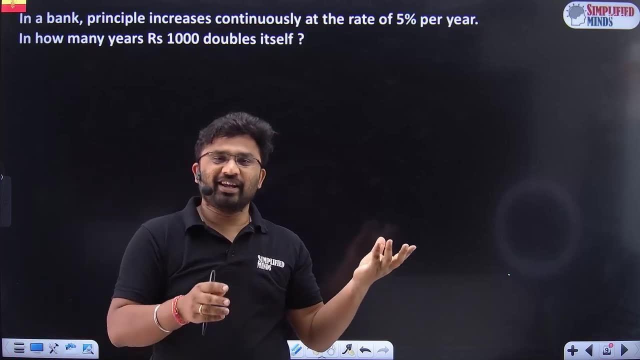 This is called. I will tell you this. You are all students, right? No one should tell you this. A simple example. This is an example. You are all confused, But most of the time. I will give you a simple example. 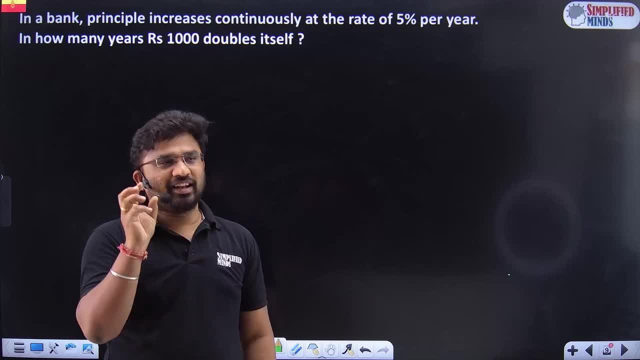 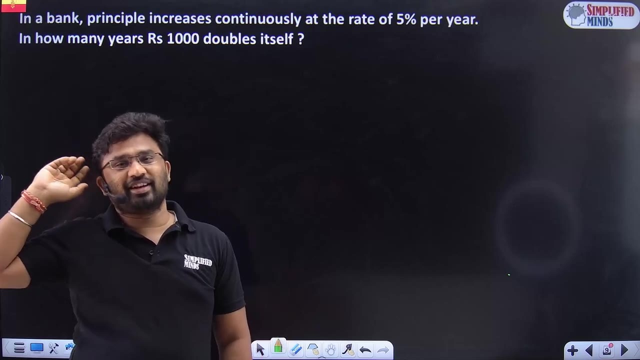 Back then I used to buy a car. I bought all the shares from that company. Now it has increased by 1 crore, I think when I bought the car the price was around Rs.14-15 lakhs. Now it has increased by 1.5 crore. 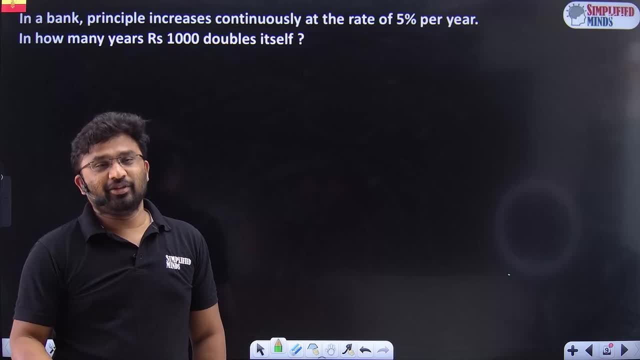 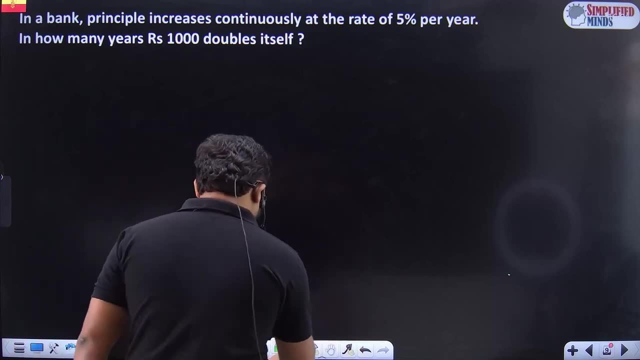 I think it is 1.2 crore, Like that. Now, when I buy a car, I buy half of it. So you have gone. So what I mean to say is, when you buy a car from a bank. see, there is something called inflation. You should know this. 5%. So when you buy a car from a bank, the value gets reduced year by year. If it is Rs.1000, you have to buy another product. Today it is Rs.1000. 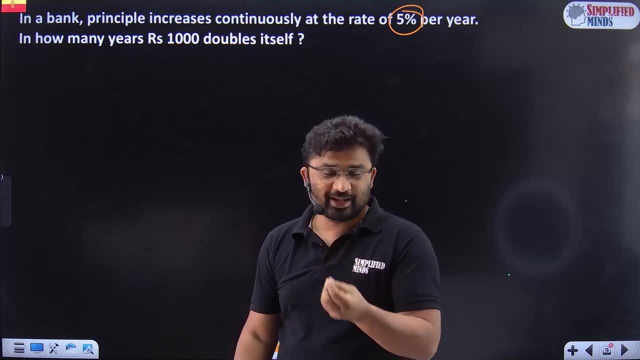 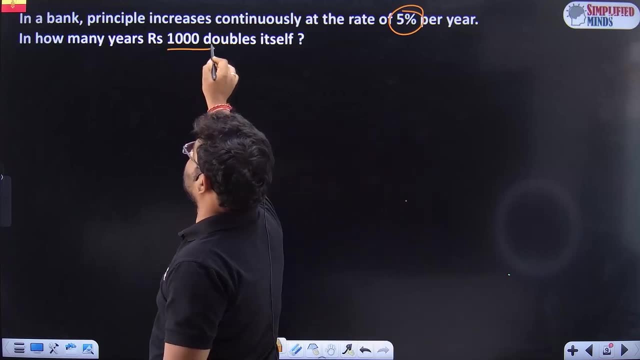 Next year it will be Rs.1050.. This is a simple example. Next year it will be doubled or tripled If you buy a car from a bank. if you buy a car from a bank, this is not going to happen. 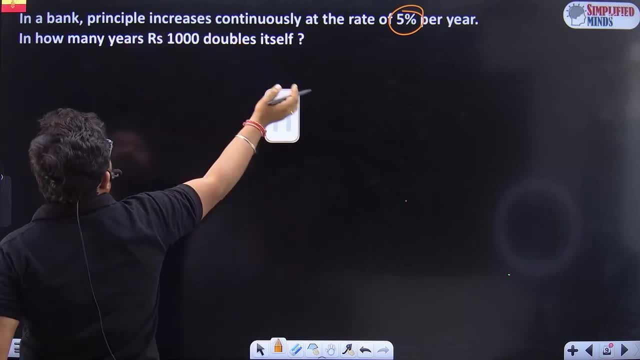 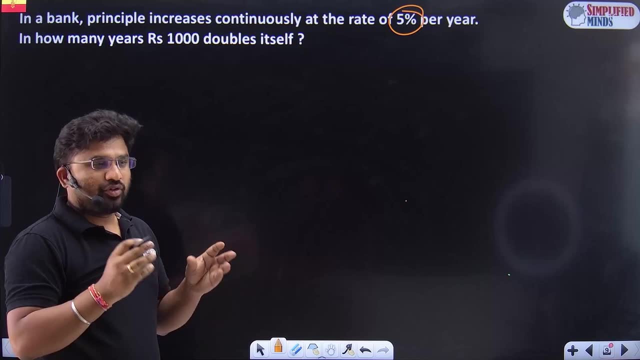 So what you are doing is while doing engineering. you should understand that the PUC is over. After the PUC is over, you have to buy a car from anyone. So you buy a car from a bank and put it in a good place. 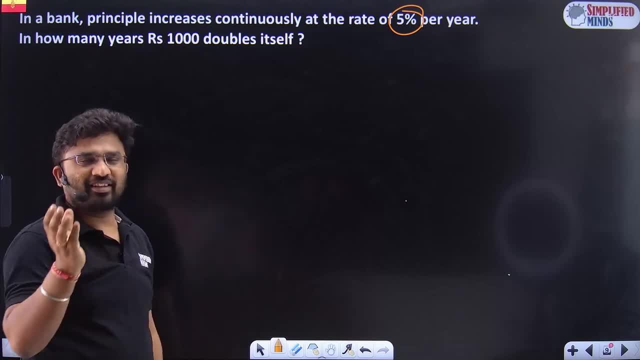 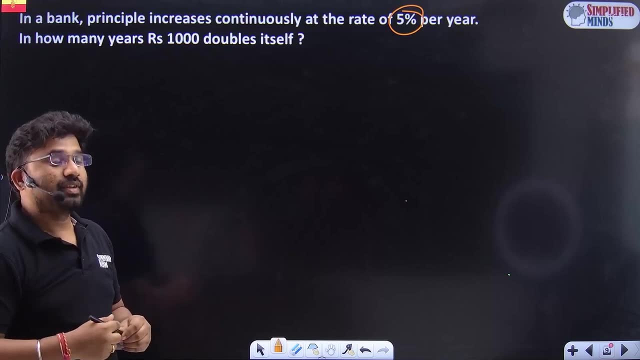 I regret it a lot. Sometimes I say I don't know anything. I don't know how to make such investments. I am teaching about shares, but I don't know how to do it. There are many people like this, So you have to study. 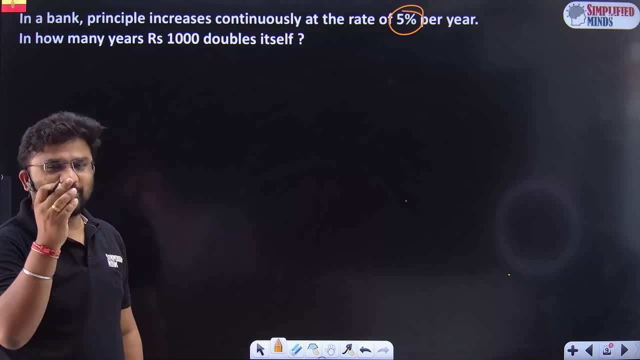 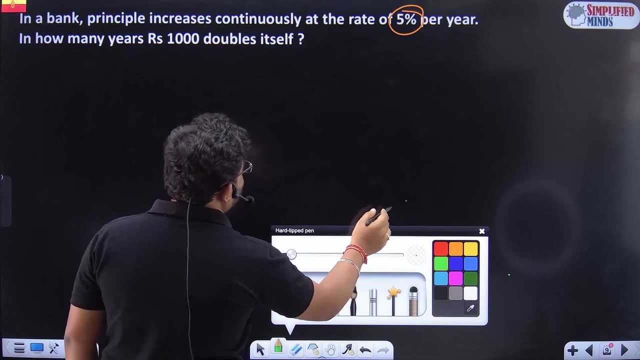 You have to understand how to do it. If you buy a car from a bank, the value gets reduced. That too, 100%, If you want inflation to be 6-7%. there are different types of inflation: Retail inflation, non-retail, etc. 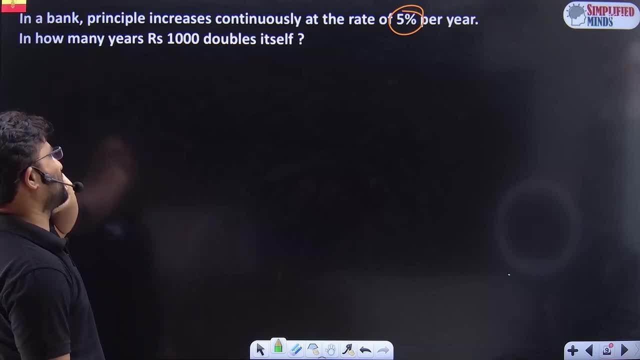 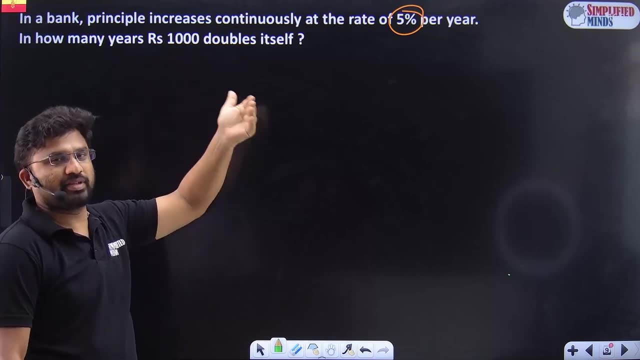 We don't need that. In a bank, the principal is continuously 5%. If it is Rs.1000, after a year it becomes Rs.1050.. In the next year you have to calculate it simply. This is the compound interest. 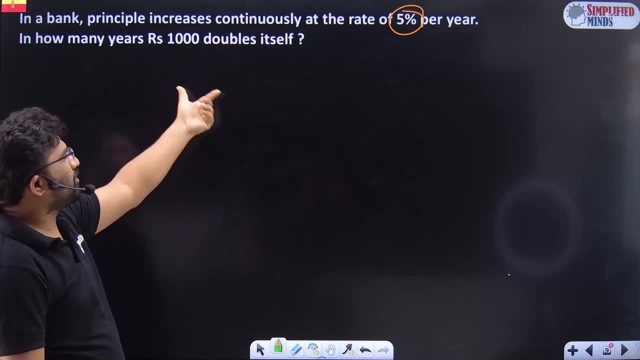 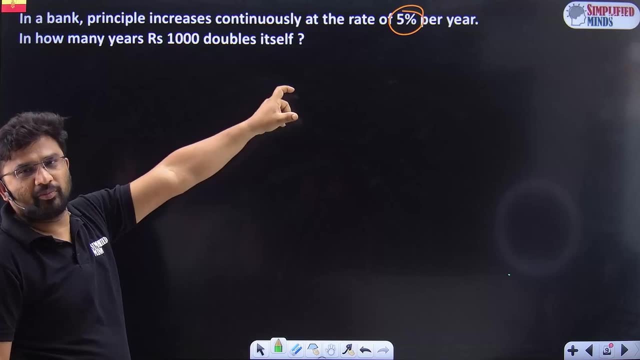 What is the simple interest? If you multiply 5% of 1000, you get a simple answer. If it doubles, it becomes Rs.2000.. Every year it becomes Rs.50.. 50 divided by 2000 is 20 years. 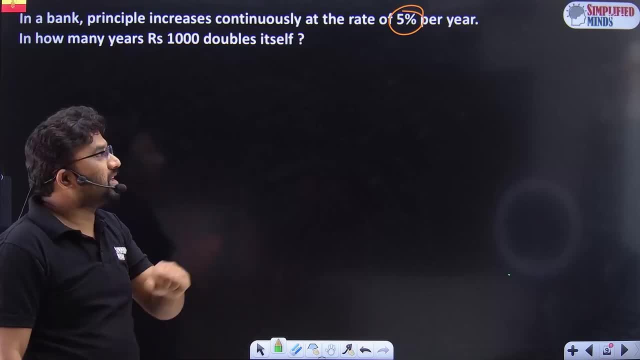 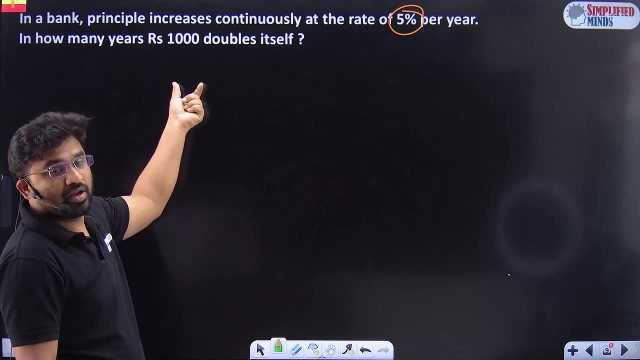 It doubles in 20 years. This is the simple interest, But this is not the compound interest. It is more than that. In a year it becomes Rs.1000.. If it doubles, it becomes Rs.1050.. In a year it becomes Rs.1050.. 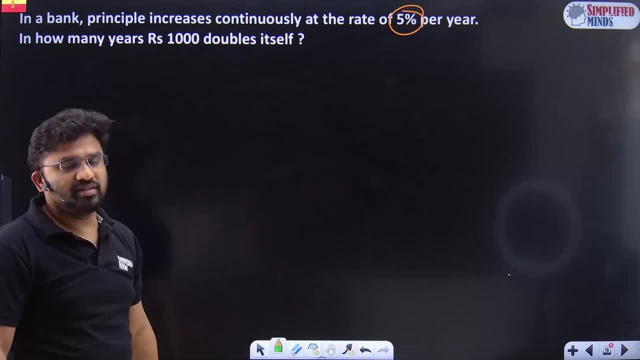 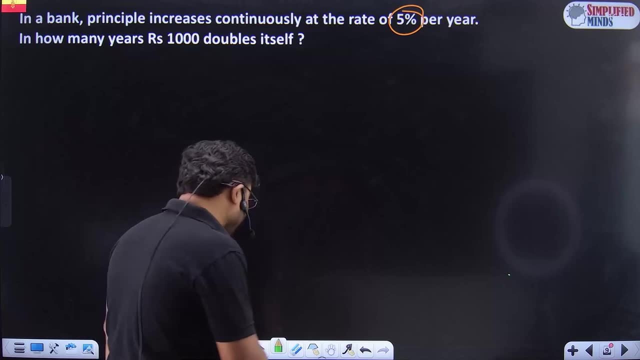 In a year it becomes Rs.1010.. In a year it becomes Rs.112.. The previous year's maturity is the principal for the next year. I am giving you the 9th class. I will come back here. I am giving you the 9th class math. 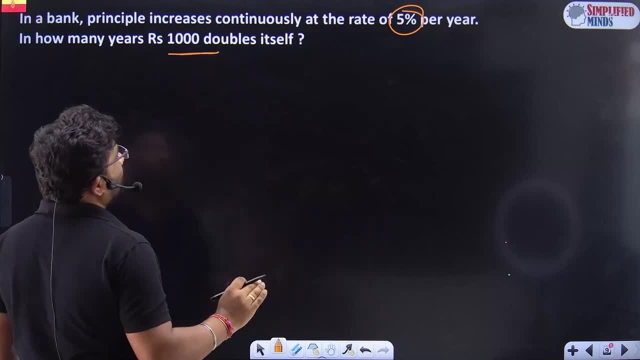 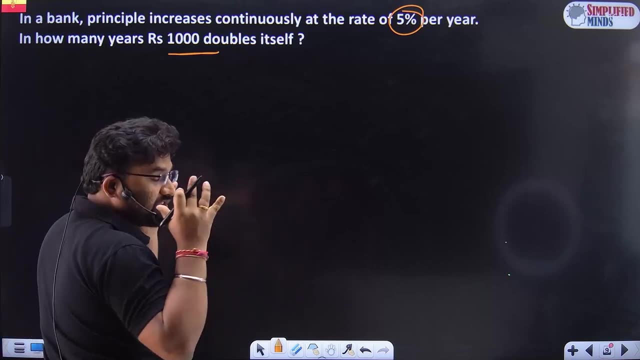 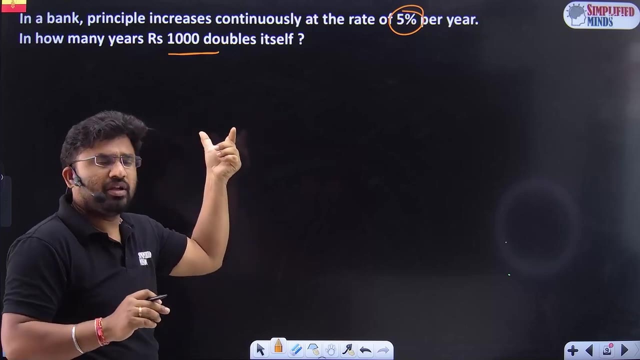 How many years it doubles. We can use the differential equation. It is very simple. This is the bank principal, What changes it makes. We can use differentiation and integration in any change In the rate of interest. in my example. we can use any calculation. 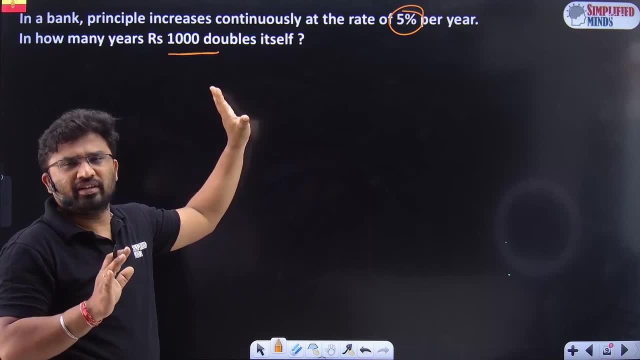 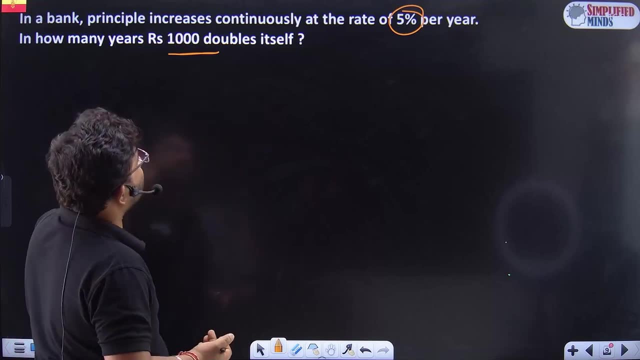 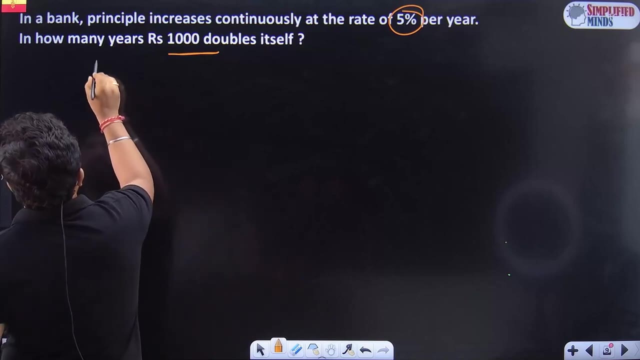 We can use it in many cases in the stock market. If you don't know, you can use the apps in the background. What changes? Interest changes? The principal changes every year. The principal is a variable. At what rate the principal is changing? 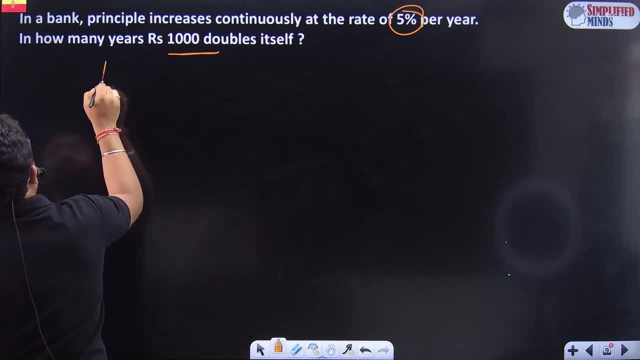 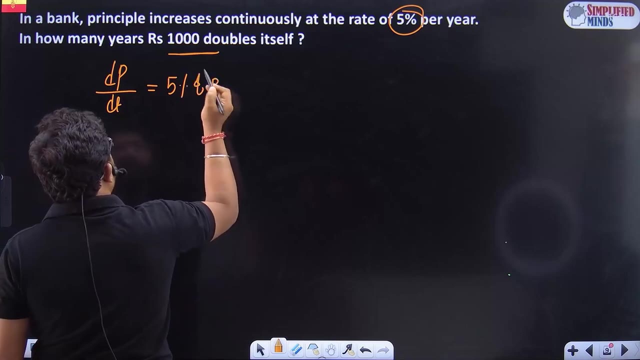 The change of the principal, dp by dt. The principal is changing. It is changing with respect to time. At what rate? What is dp by dt? It is changing every 5%, 5% of what Of p. This is the equation. 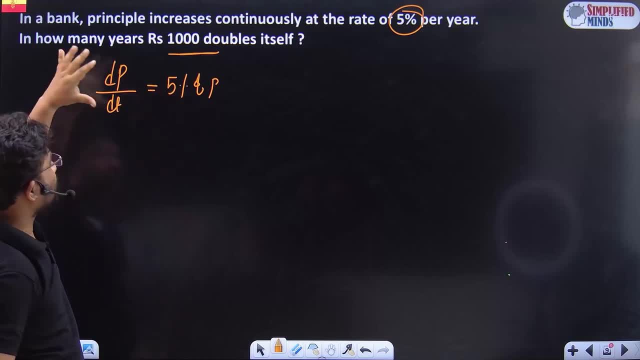 dp by 5% of the principal. How much does it change every year? The rate of change is 5% of p. If it is 5% of p, it becomes constant. 5% of p. After that, dp by dt is 5% of p. 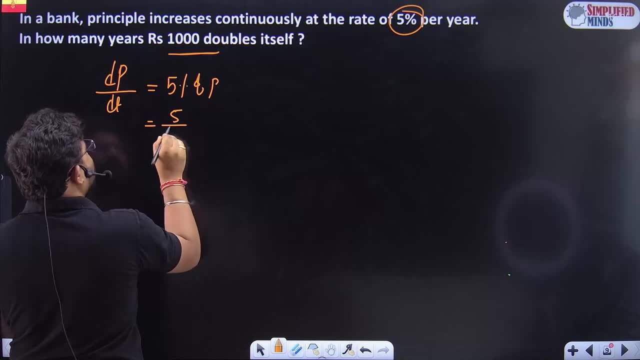 This is 5 by 100. It is 1 by 20.. 5 by 100 p, That is dp by dt. After that you have to integrate and get the value of p. They have given a smart boundary When you put the first time bank. 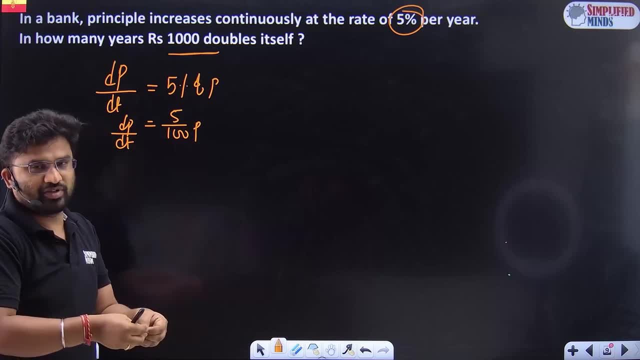 time is 0. But you have taken it. Why did you take 1000 rupees? In books, people should teach rich things. We are keeping 1 crore in the bank. Everyone asks for 1000 rupees and 100 rupees. 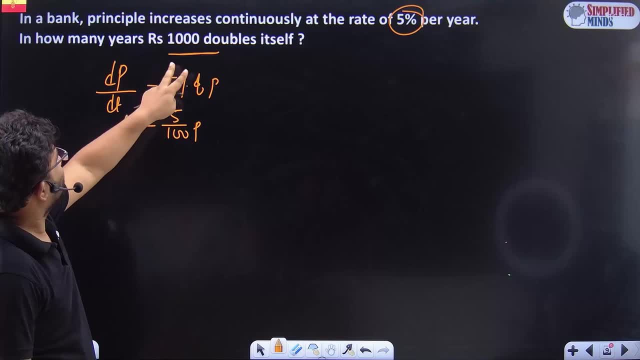 Let us change it. It is not 1000.. Rupees is not 1000.. We will make crores, 1000 crores. We are Ambani's. Let us keep 1000 crores in the bank. Our thoughts should be rich. 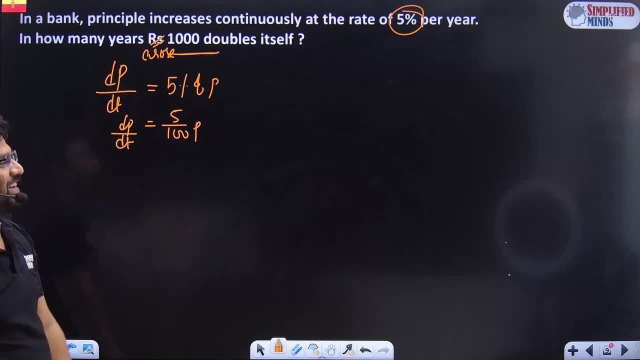 If we are not rich, our thoughts should be rich. 1000 crores in the bank Next. dp by dt is 5% of p. How much is 5%? It is 1 by 20.. I take p by 20.. 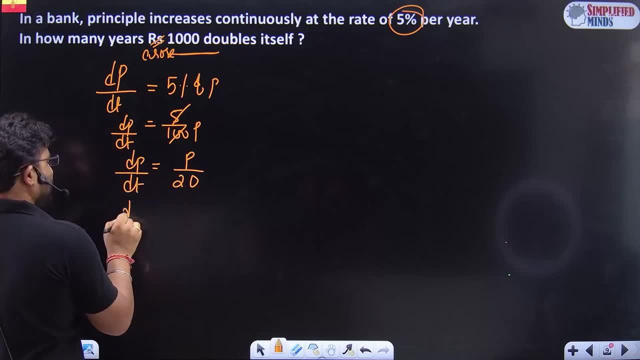 dp by dt. It is difficult to integrate. Variables are prayable. dp by b is equal to dp by 20.. Integrate and it is very simple: Log p. If you have problems like this, integration is very easy. This carries marks. 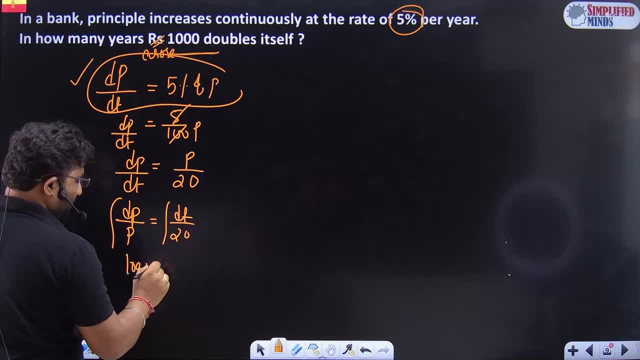 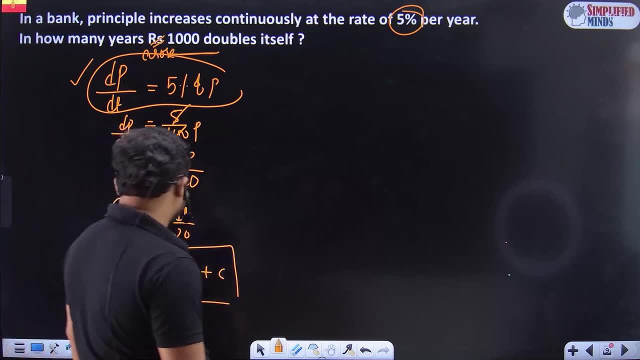 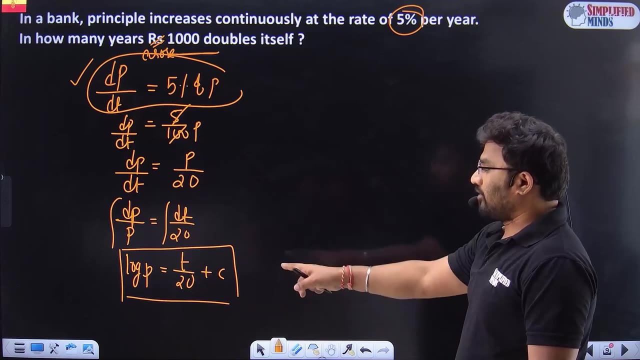 Thinking this integration of 1 by p, log p is dt by dt, t by 20 plus c. This is the equation. Look, Log p is equal to t by 20 into c. I have to put now: Log p is equal to: 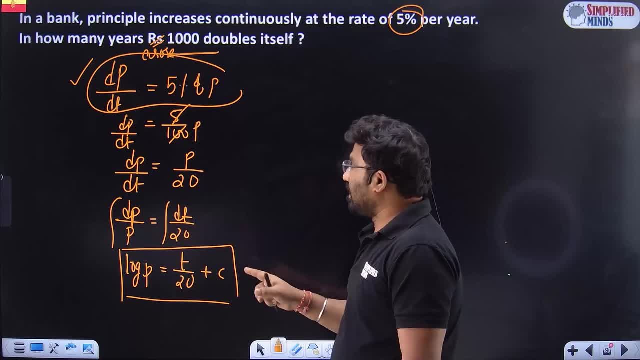 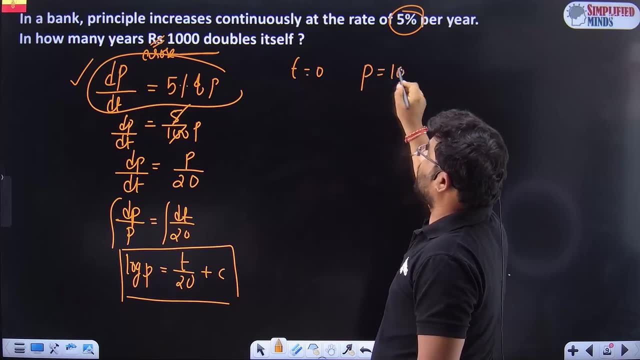 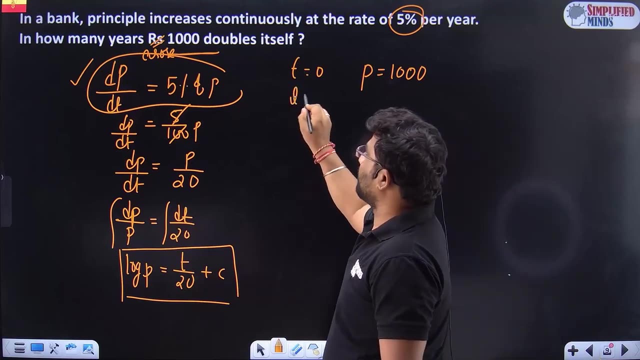 t by 20 plus c. What is the question is asked is time is initially 0. Condition: How much is the principal? 1000 crores, 1000 crores, 1000 crores? What is the time? 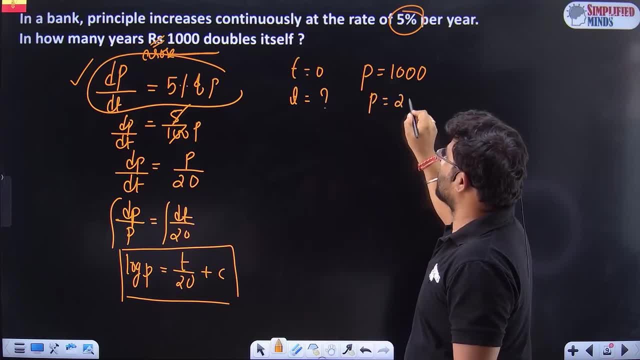 We don't know. My principal becomes 2000 crores. Ok, Next, When I substitute log p, I have to get the value of c. Use the first condition, 0 comma 1000.. In the previous question I have given x and y. 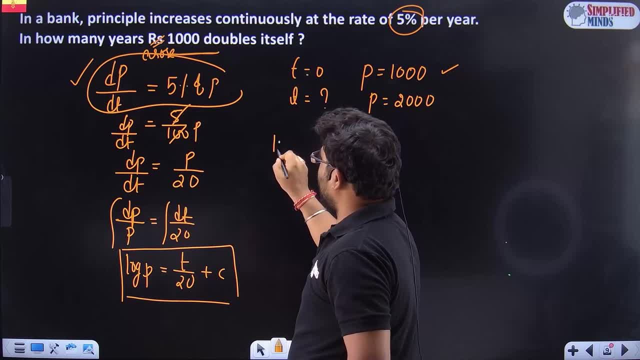 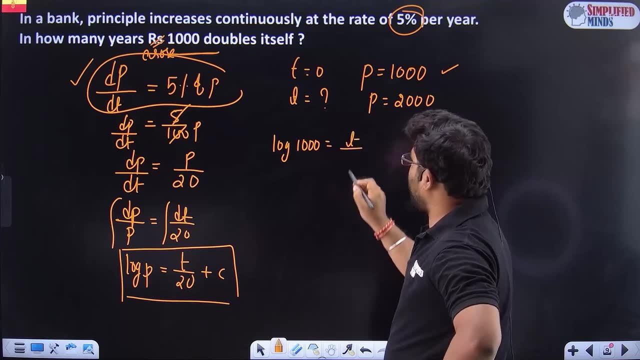 I have given t and p. Put t in this equation: Log 1000 is equal to p. What is t now? t divided by 20.. Next is 0.. 0 by 20 is 0.. c is 0.. 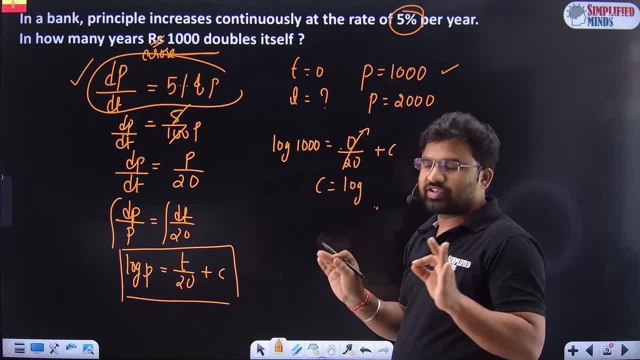 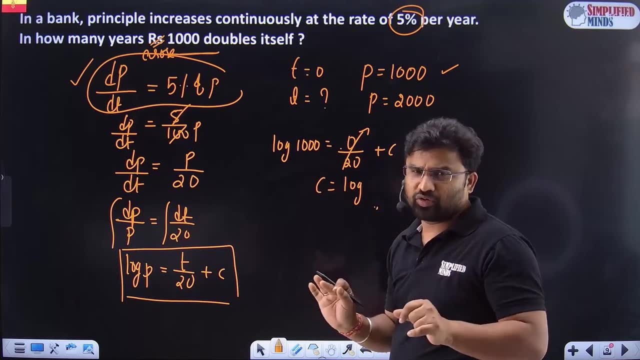 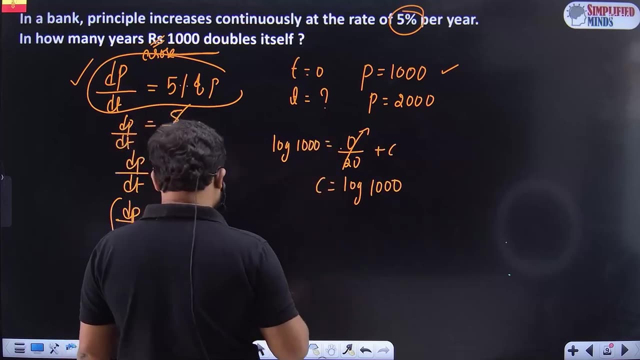 c is log By default. I have not mentioned anything. Log is not a base. It is a base When we come to log. it becomes a base When log is 1000, we get the c value. Now our equation is updated. 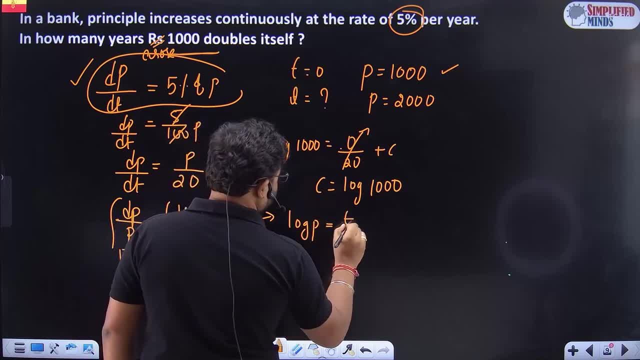 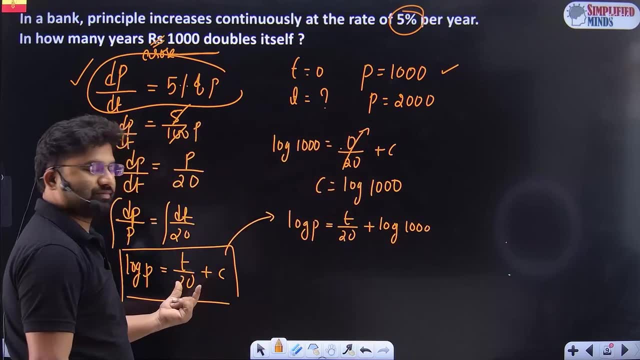 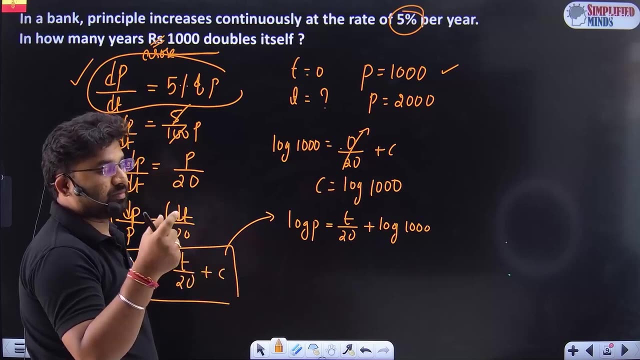 as log p into t by 20 plus log 1000.. This is a particular case. This is general. Now what is the value of p In physics, if you remember the derivation of the nuclear law of radioactive decay In chemistry? 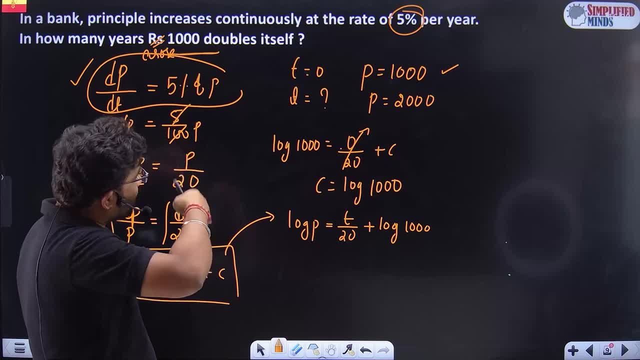 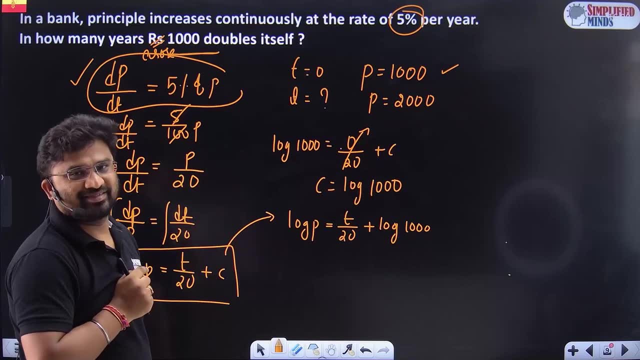 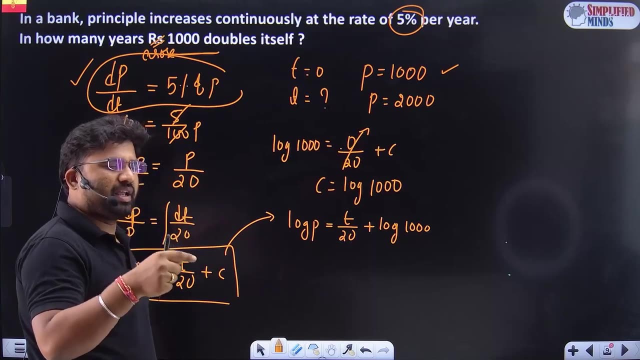 there is a rate derivation. It is a first order derivation. Do you remember? t plus t is equal to 0.. r is equal to 600.. I think you remember this. t must be equal to log p 0, 3 divided by. 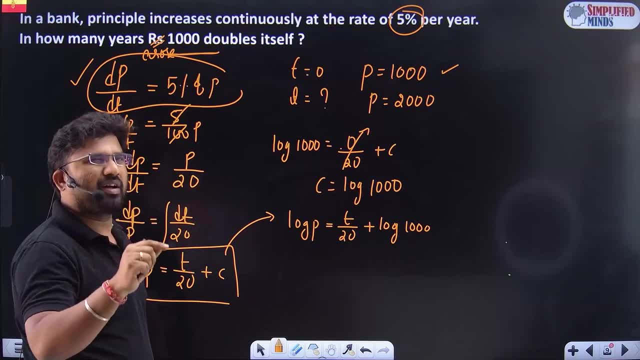 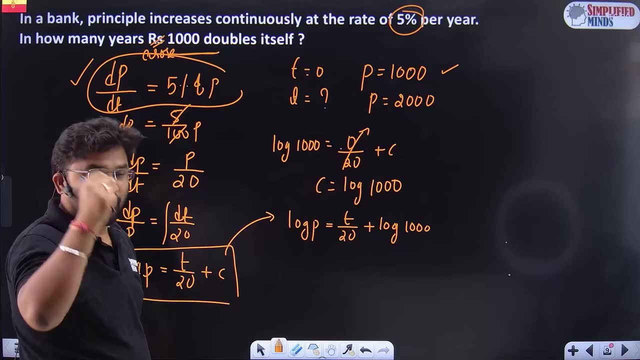 t into log of r by r 0.. r 0 by r 0 is equal to. t is equal to 2.32 by k. k is equal to the first order derivation. This is the same derivation. log p is equal to. 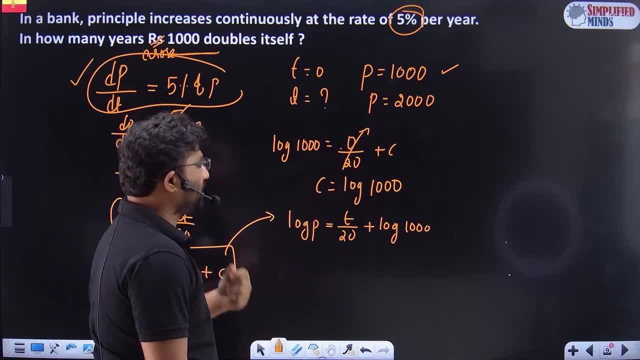 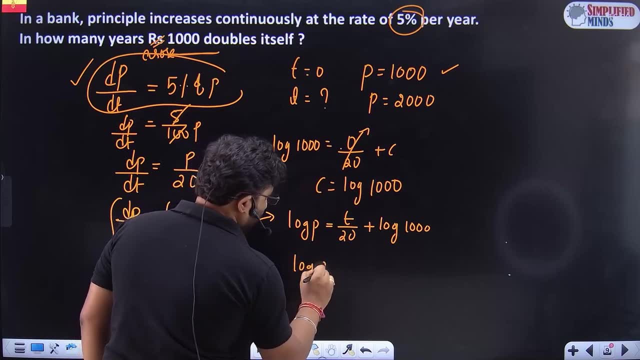 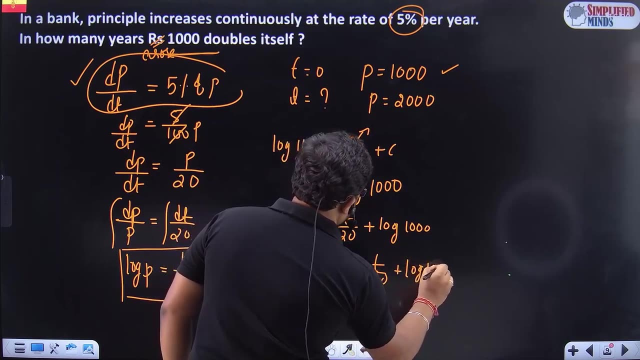 t by 20.. What is the value of t for which the p becomes 2000? When p is substituted by 2000,. log 2000 is substituted. We get t by 20 plus log 1000 cross When this is substituted. 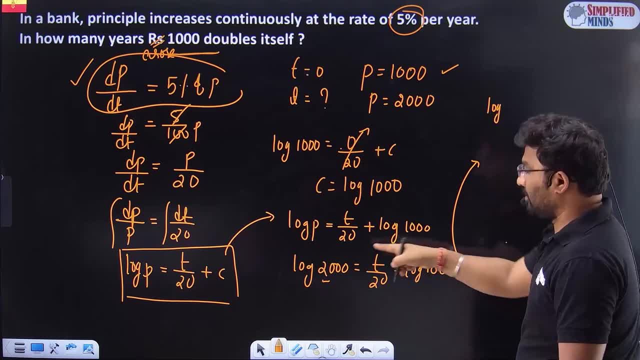 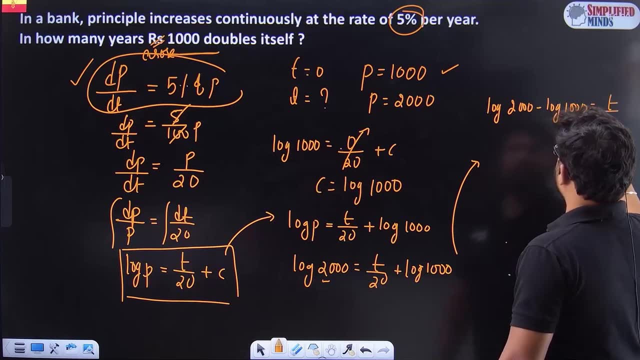 we get log m minus log n. log m minus log 2000 minus log 1000 is equal to t by 20.. log this by this is 2000 divided by 2000 by 1000.. That is nothing but log 2.. 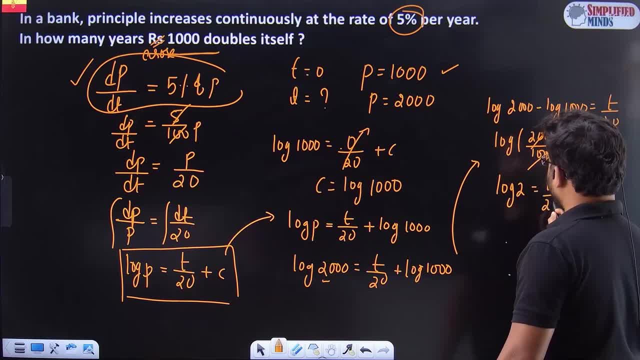 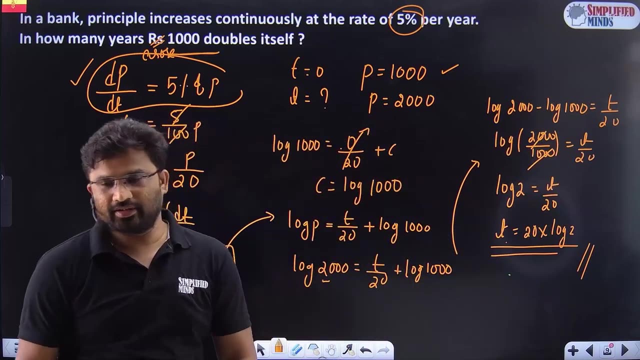 log 2 is equal to t by 20 and the time is equal to 20 log 2.. This is the answer. Again, you can substitute log 2 and get the answer. I will get the calculator. I will give the exact answer. 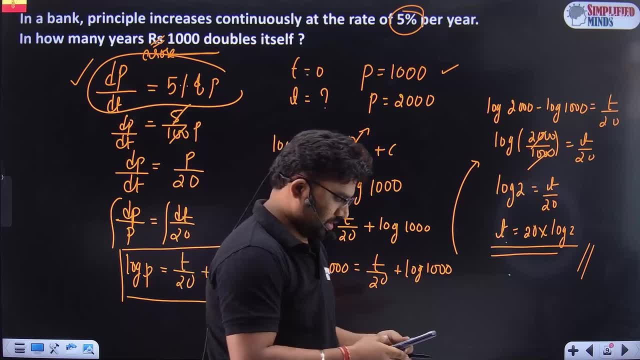 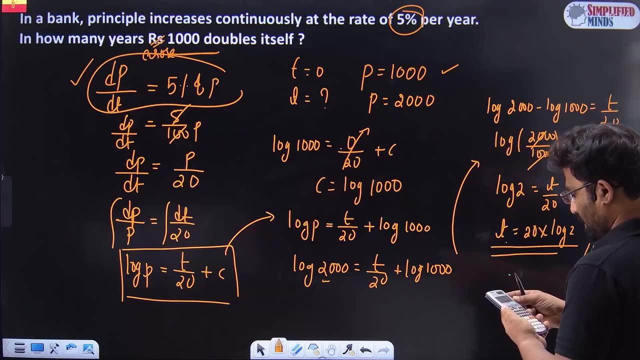 So log 2 into log 2 minus t by 2, t by 2. this is the fathering of the equivalence. stop, take the theoretic order way. It will be equal to t by b, being equal to t by 2, t by b. 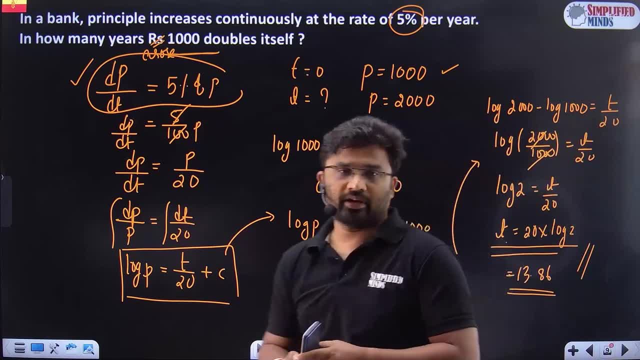 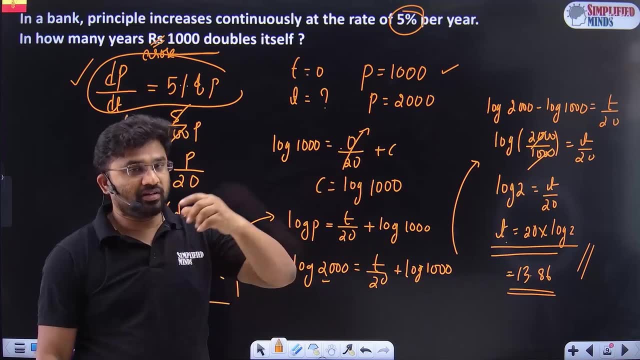 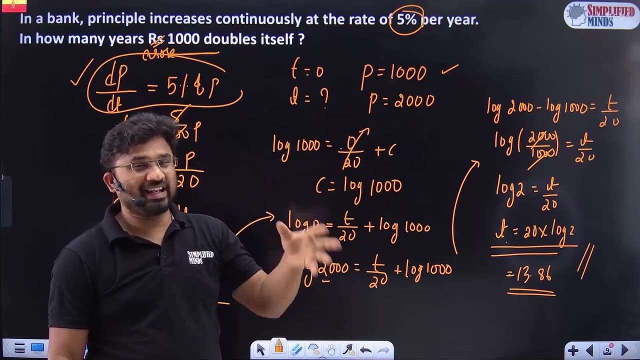 If sorry. D by dollar is equal to t by a. 1. you is women, wes. 0, 7 years have passed. Imagine you have 1000 crores In 3 years. you have 1000 rupees as your value. 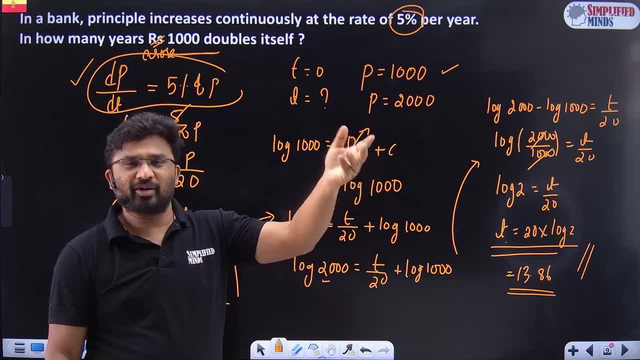 If you want to buy a property, you will become a big business man. You will be like a teacher. If you want to buy it, it will be 5000 crores, Even though 1000 became 2000,. by the time, 20 years gap. the price of the property will be almost 3 times or 4 times. So there is no point of putting in the bank If it is double to 5% in 13 years. you know that in stock markets usually 12%, 15%, some even take 30%. 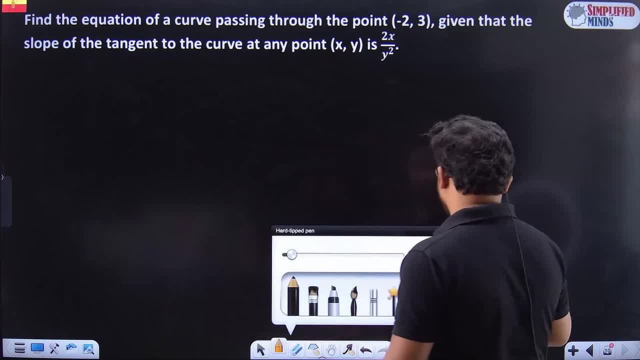 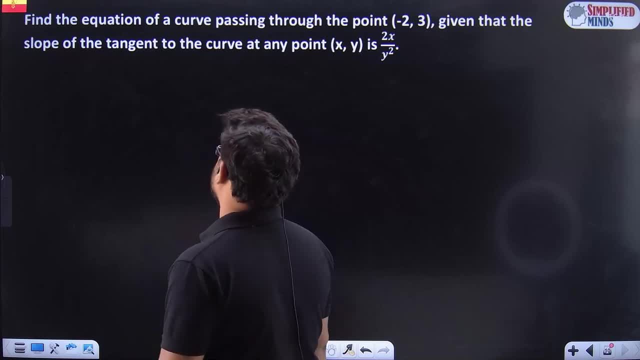 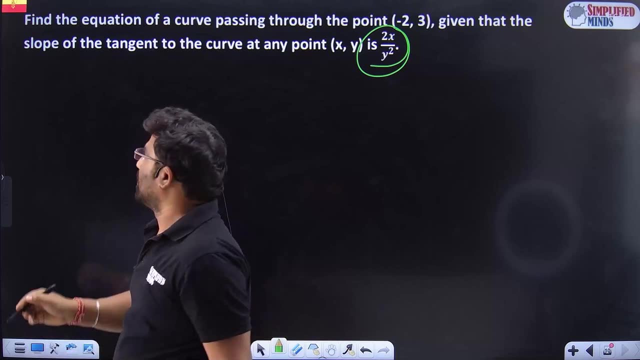 Find minus 2,3. given that the slope of tangent of the curve is given at any point, is this much? Slope of the tangent. Slope of the tangent is dy by dx, So dy by dx, dy by dx is equal to. 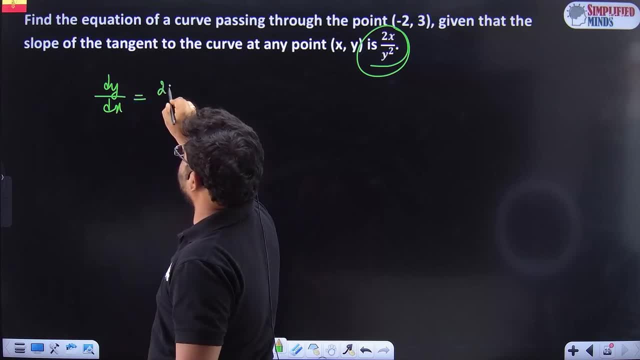 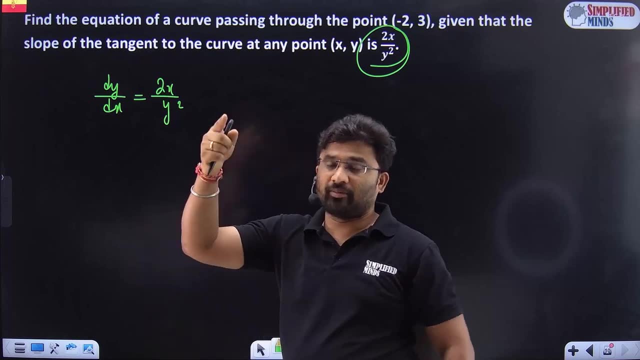 2x divided by 2x divided by y square. So we have already done maths. You can see that there is an application derivative of slopes and tangents. We have deleted that right. So this problem will come here So we can ask what is needed in maths. 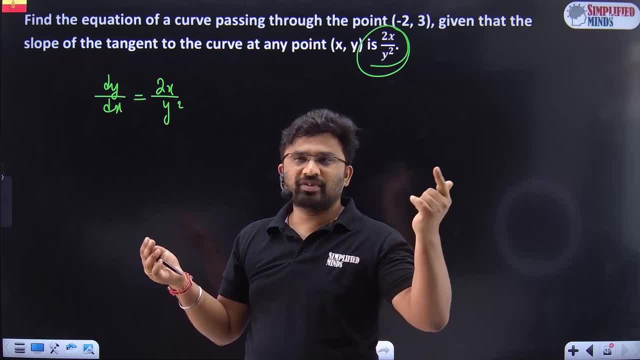 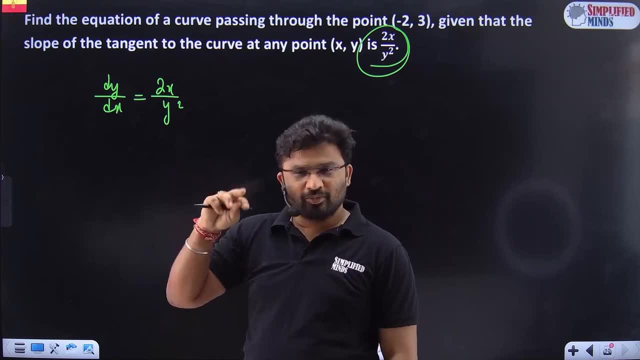 We have already done a few new ncrt. There are no slopes and tangents here. There is an application derivative in differential equations. We can ask here right. So slope of tangent is normal commonsense. So no need to delete that portion. 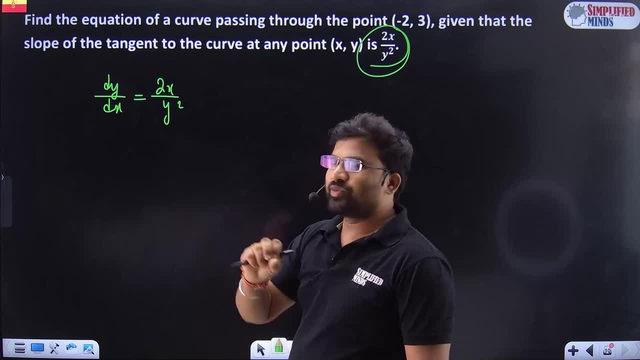 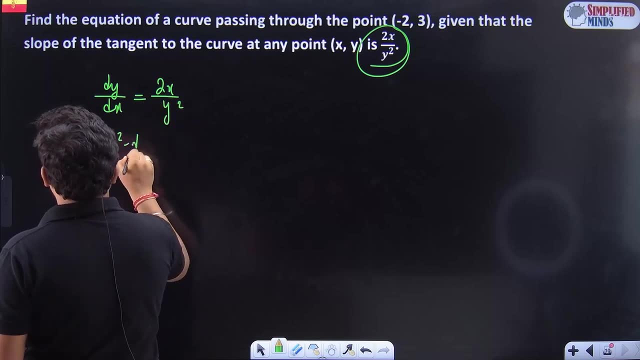 Then the question is CET also. Next, dy by dx is equal to 2x. divided by y square, Again same thing. So shift here So you will get like y square into dy must be equal to 2x into dx. Integrate that, So y square, integration, y cube by 3 and integration 2x. 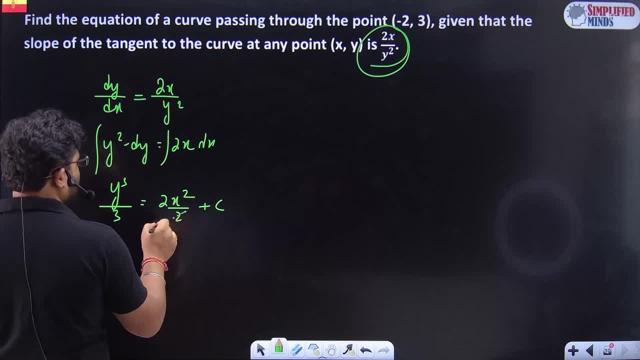 square by 2 plus c, So 2. to cancel, I need to find minus 2 comma 3.. So y cube by 3 is equal to x square plus c. After that I need to find y cube in y place, So we get the. 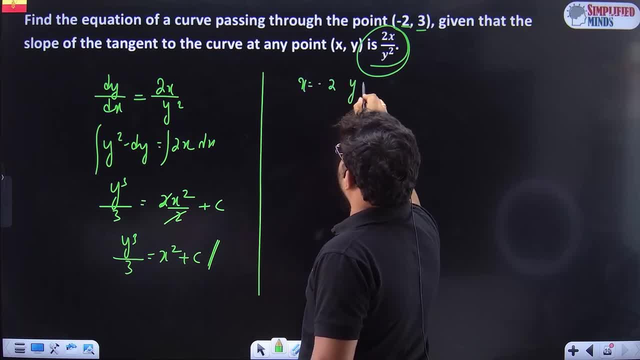 value of c. Substitute x as minus 2. y becomes 3.. So minus 2 is substituted 27.. 3 cubes are 27, divided by 3 should be equal to 9.. No, not 9.. Minus 2 square 4 plus c: How? 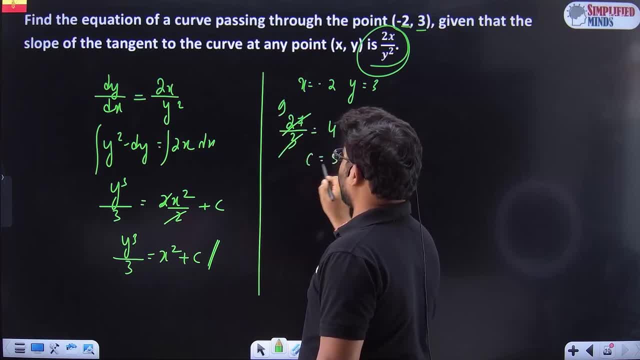 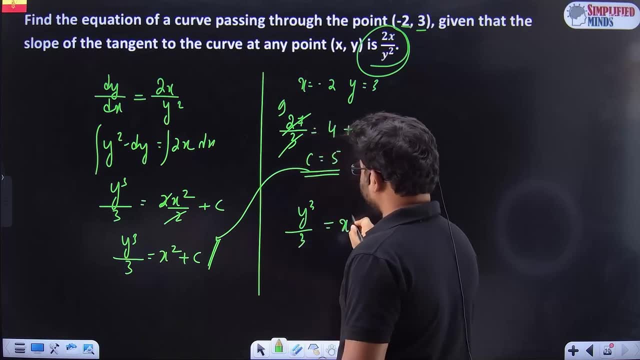 much 9, right 9.. So c must be equal to 5.. To substitute this, so we get the value of this solution In particular, equal solution: y by 3 plus square plus 5 comes out here. 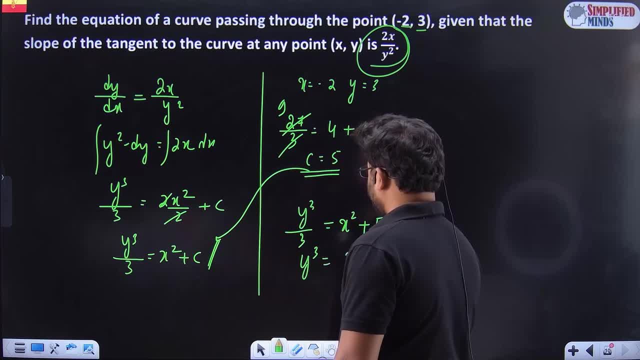 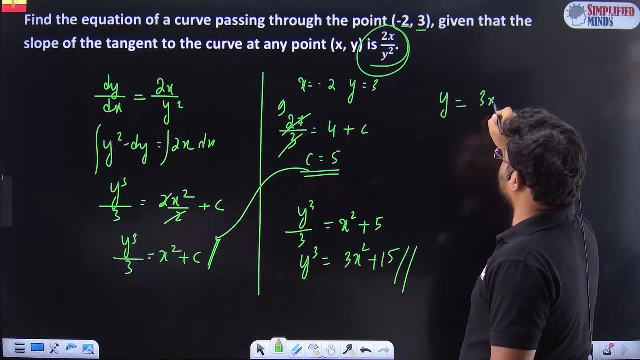 So y cube is nothing but 3x square plus 15.. If you want y in the form of y means you have to get 3x square to the power of 15, to the power of 1.. Simple children, So variable. 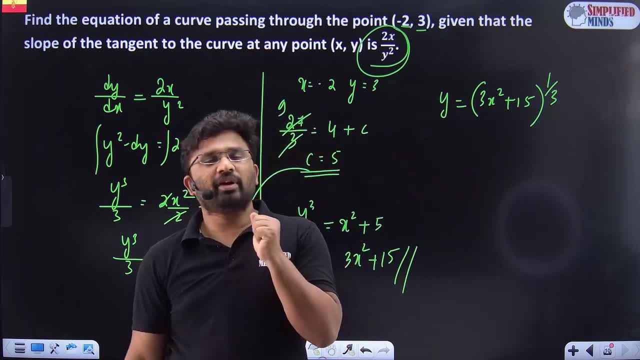 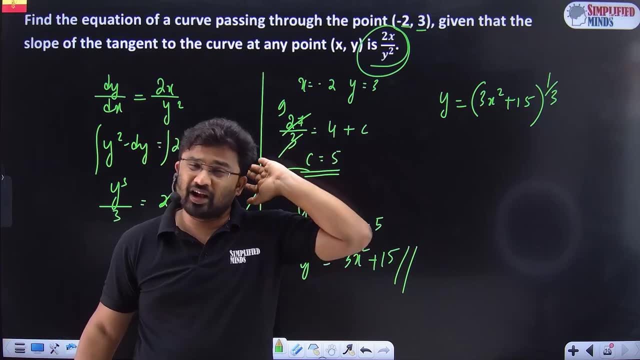 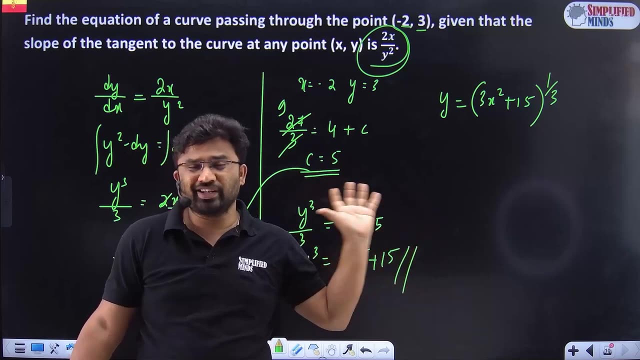 separation is a very easy method. See, now you have to separate your other questions by using the variables. So after that, So you have to integrate. You can ask any tough question in this. So how good your integration is. but PUC board exam point of view, what I am teaching is very good. This is more than sufficient. 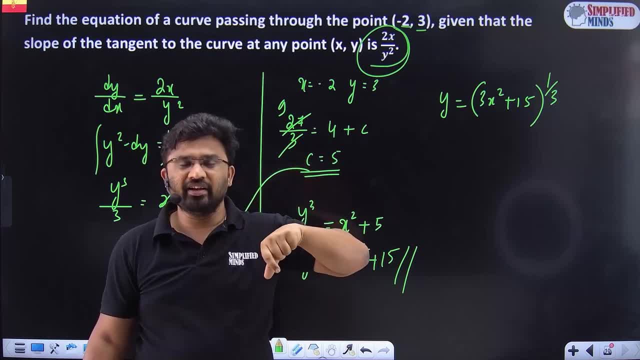 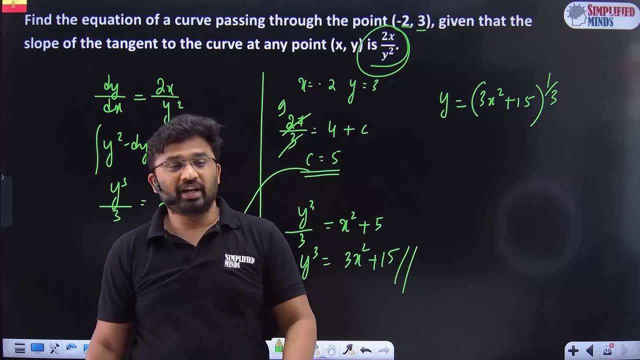 So integration will depend on it. The more complicated the integration, the more complicated it will be, For example, in homogeneous questions. the more integration we get, the more complicated it will be, Because we get the quadratic equation terms in homogeneous. 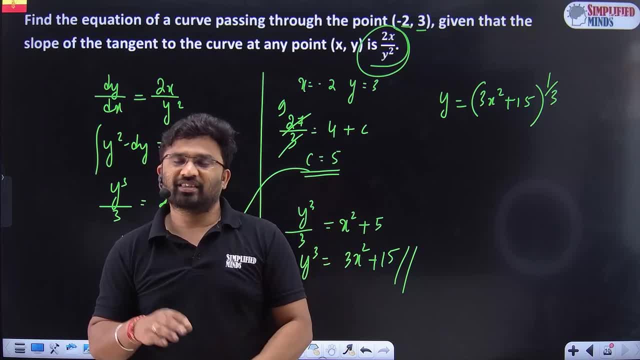 So it is very easy. We will do that. questions also, And I hope you understood this. So don't forget to comment: not integration, but calculus is love. Integration is over already, And that's it, my friends. See you in the next videos. Bye, bye, Take care. 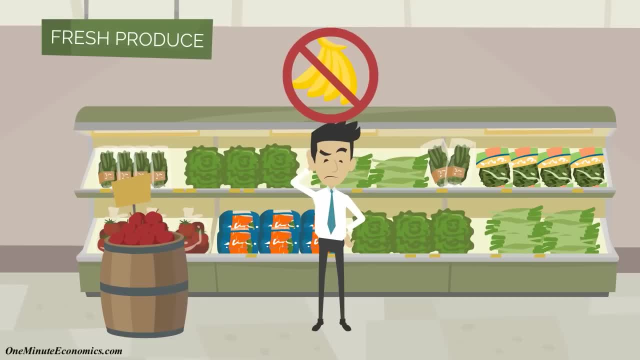 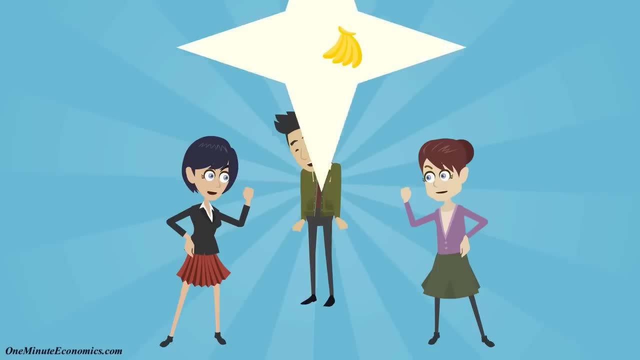 Let's assume you live in a small town where nobody sells bananas. In other words, zero supply. Now let's also assume that the people who live there would love to eat bananas. In other words, there's a decent demand for bananas. 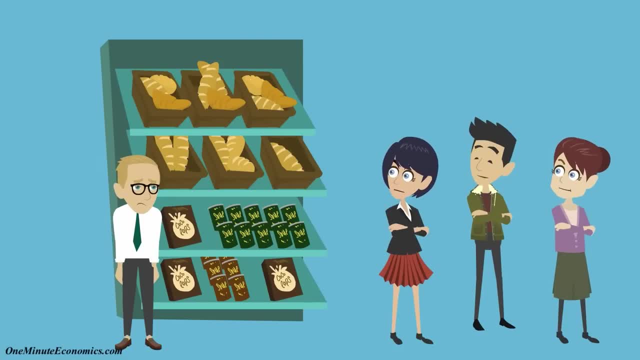 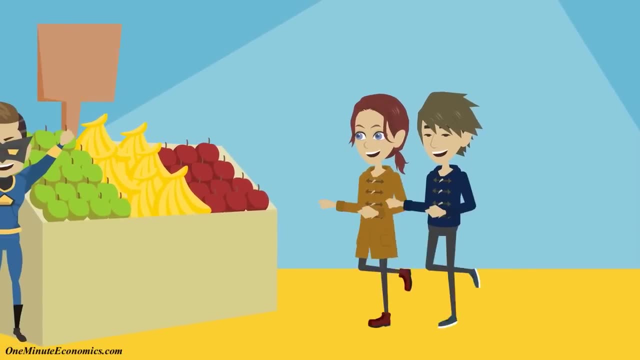 As we can see, there is currently an imbalance. People want bananas, but there are no sellers. Peter understands this and starts selling bananas At the beginning. his profits will be huge because lots of people want bananas and he's the only one who has them. 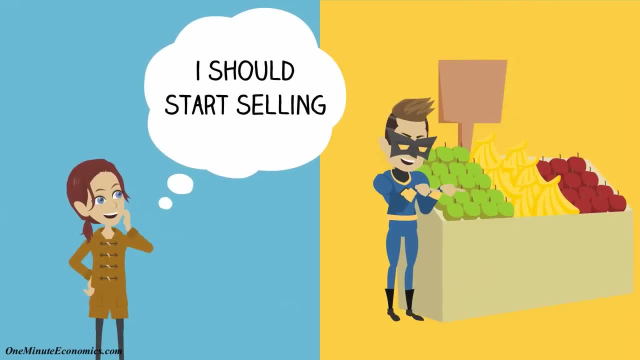 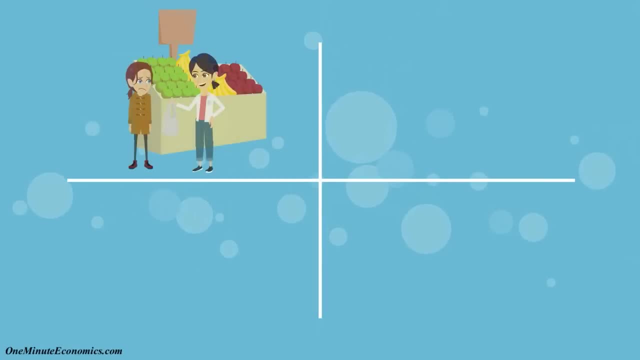 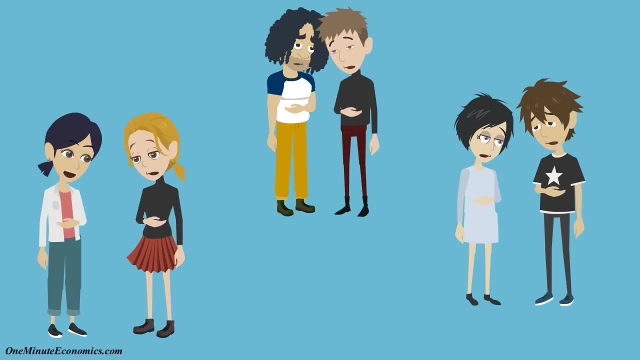 As time passes, however, Sarah will notice how well Peter is doing and starts selling bananas herself. This increases the supply of bananas and diminishes Peter's profit potential. The more people start selling bananas, the more supply there will be. If too many people end up selling bananas but the demand doesn't increase as well, there will be too much supply and some of them will go out of business.